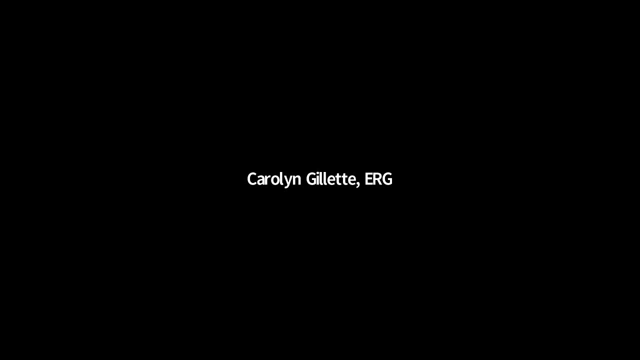 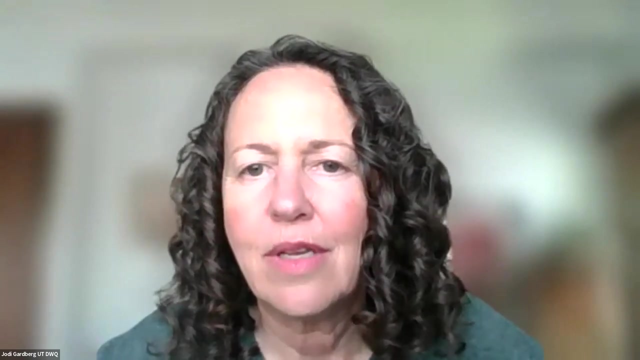 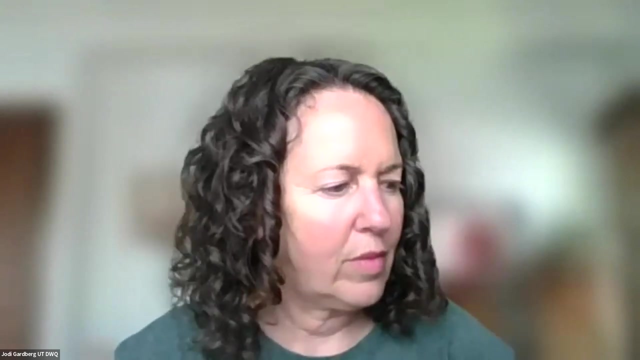 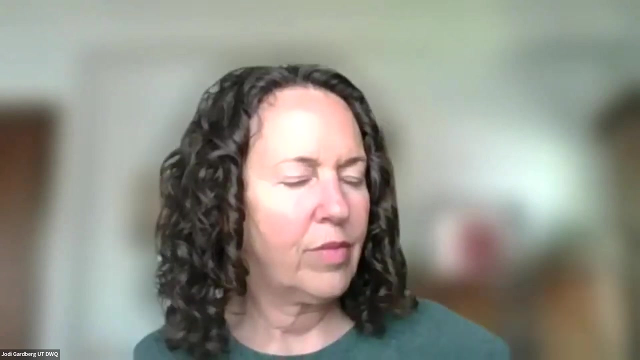 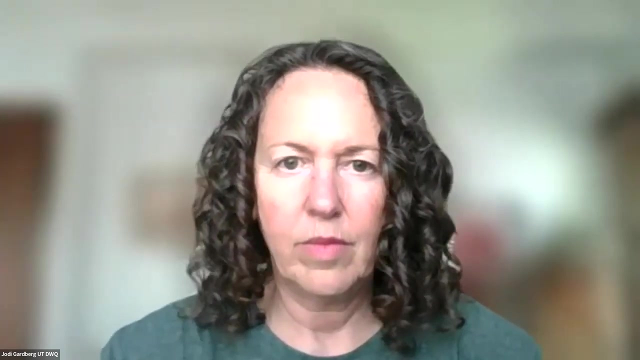 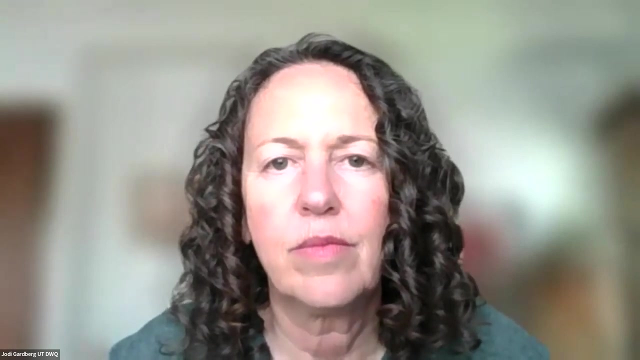 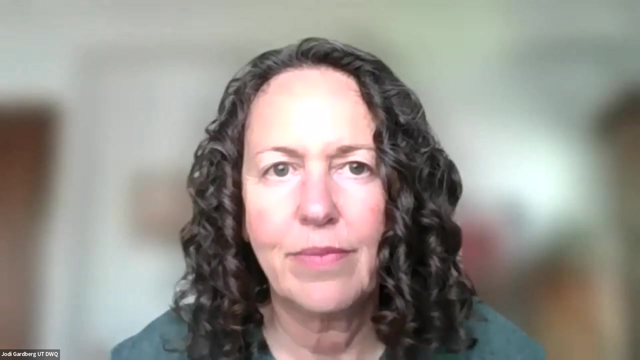 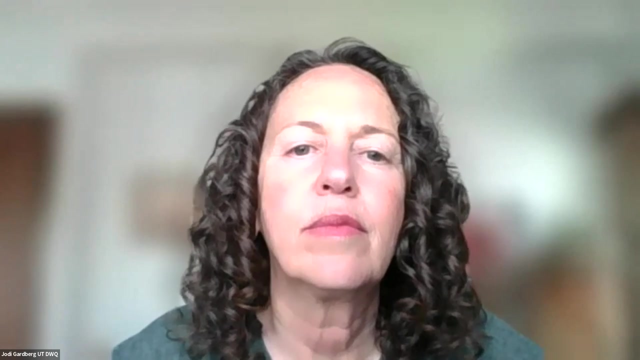 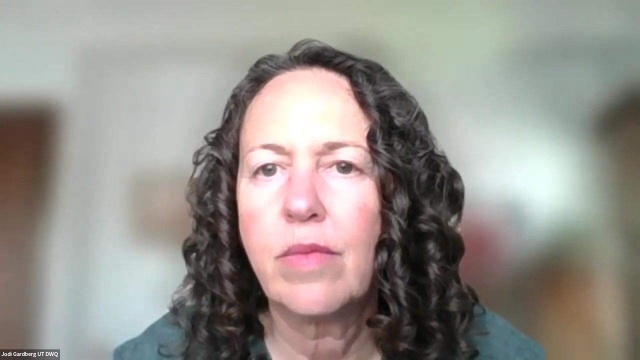 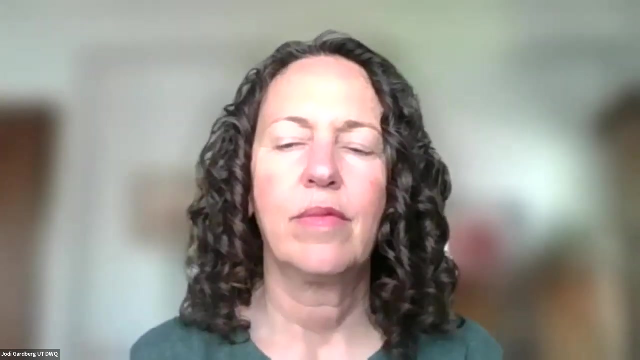 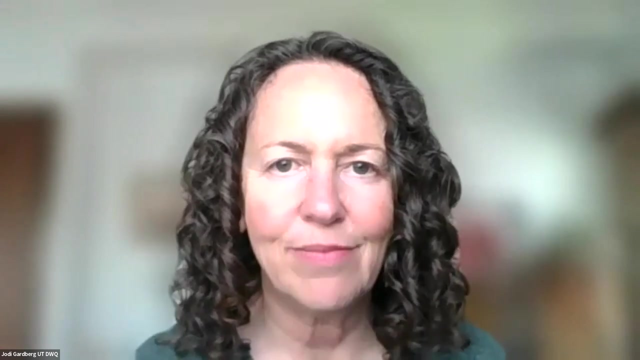 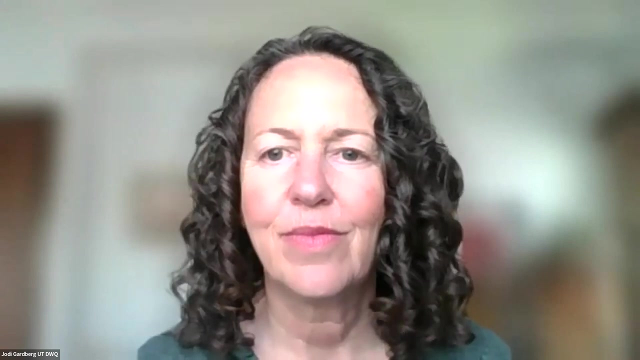 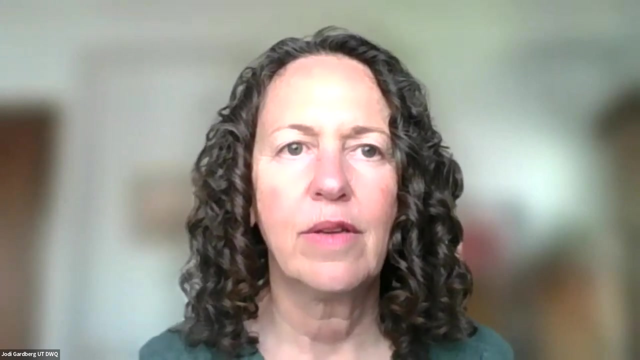 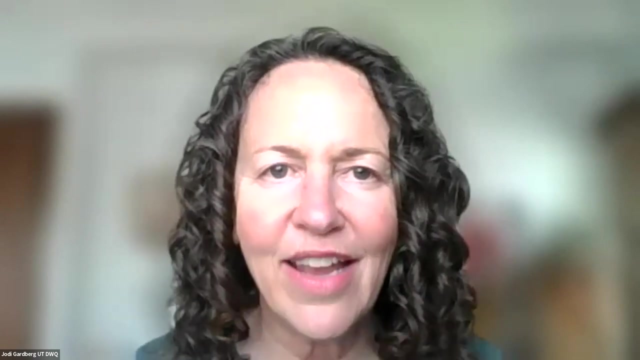 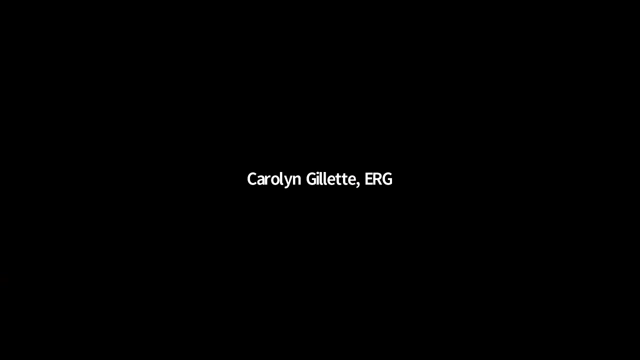 Thank you, Hi everyone. Thank you for joining the Lunch and Learn. We're just waiting a couple more minutes to begin. Hi everyone, Hi everyone. Is it now good, Carolyn? Yeah, I think we'll probably get a few more folks, but nobody else is in the waiting room. 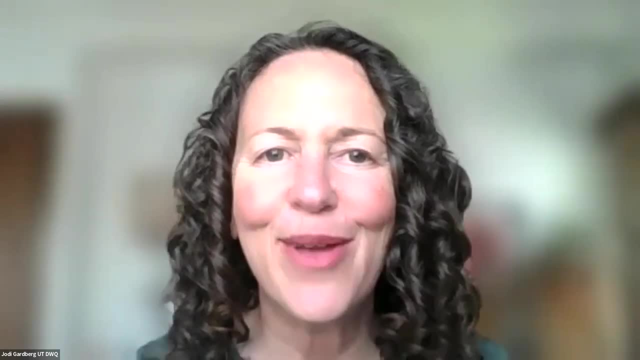 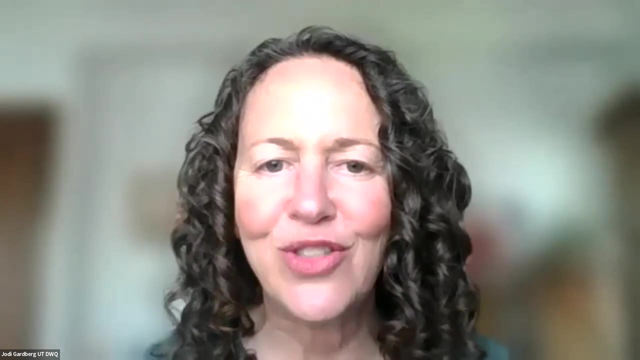 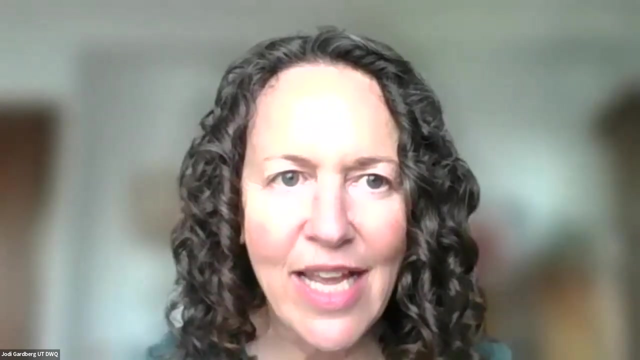 Okay, perfect, Welcome to the Lunch and Learn. I am not Christine Osborne, I'm Jodi Garberg. I work for the Division of Water Quality. I manage the Watershed Protection Section. I think I've met most of you. We have a great presentation today by Gigi Richards. Richards, right, Richard. 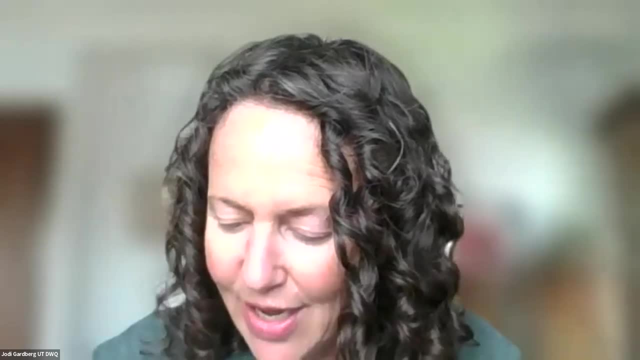 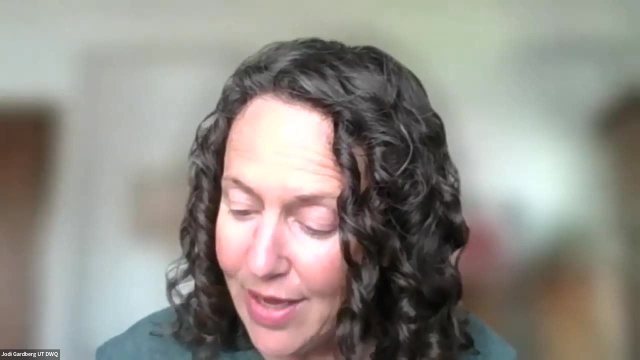 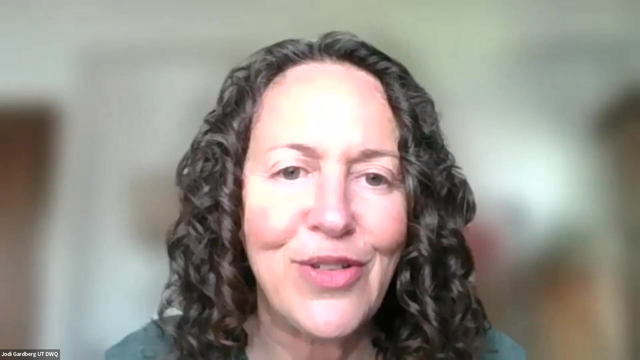 Gigi is the director of the Four Corners Water Center and she also teaches geosciences at Fort Lewis College. She's going to talk about snow and watershed monitoring in the Animas Basin and geomorphic monitoring of the Dolores River. So super excited to hear Gigi today and to see all of you here. 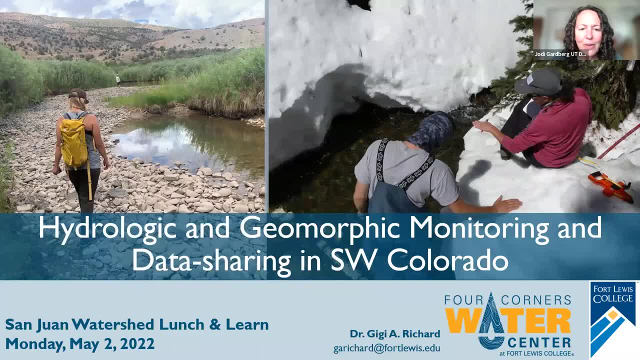 She's going to share a presentation. I'll just remind people that this is being recorded so you can see it later on. And then also you can use the chat function for questions, or you know, I don't know Gigi. 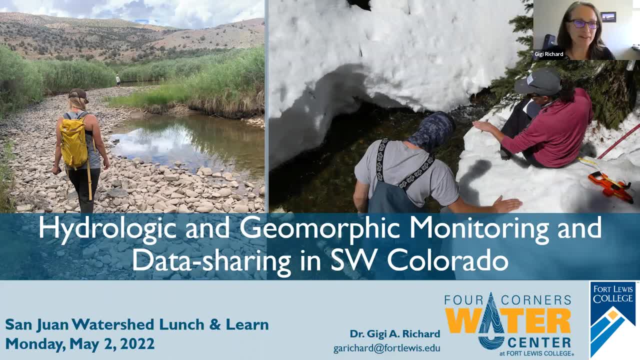 do you take questions during your presentation? Yeah, that'd be great. Yeah, okay, Well, take it away, Gigi. Okay, thank you, Awesome. Thanks, Jodi, And I just want to check in. Are you all seeing my PowerPoint? 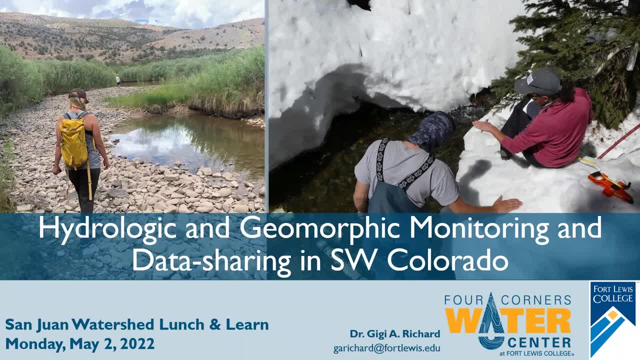 Yes, Okay, great, Awesome, Thanks. Oh, do we just lose Gigi Froze up? Oh, no, Gigi, you're frozen. I'll send her a note in the chat as well. Okay, I don't know if she knows. 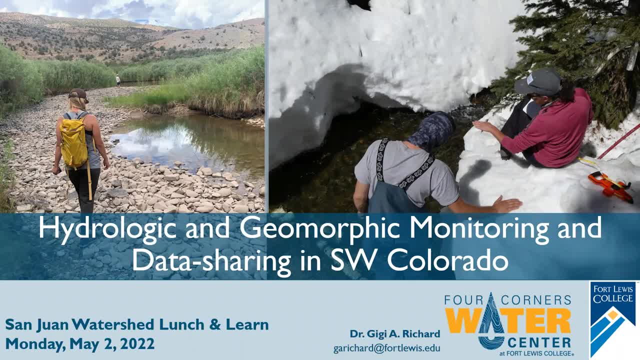 I definitely can't give this presentation in her stead. Maybe Just send her a note. I'll see if she can log in and out again. Yeah, either that or call in, maybe, And we can also. I can also run the presentation for her too, if that's. 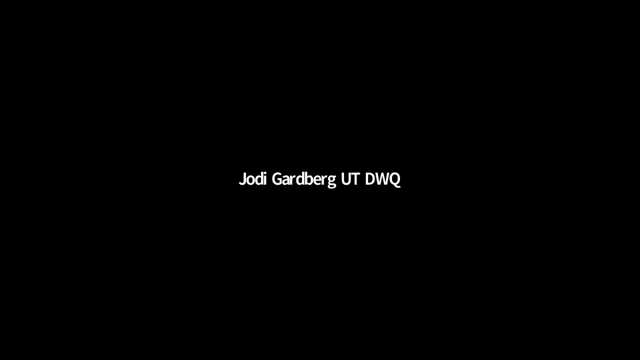 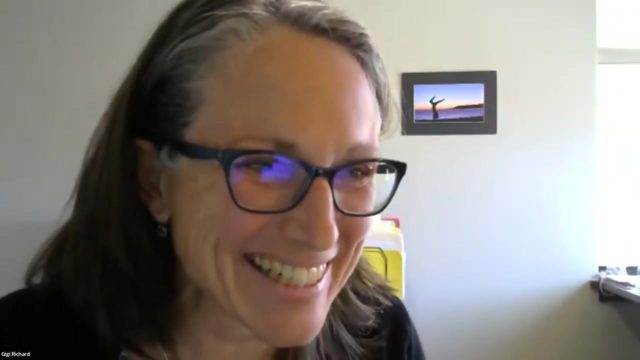 Okay, good, good, good, good. So please stay on the line. Okay, we can see you. Okay, good, good, good good. Internet just went out. Bad timing. Yeah, All right, We'll try this again. 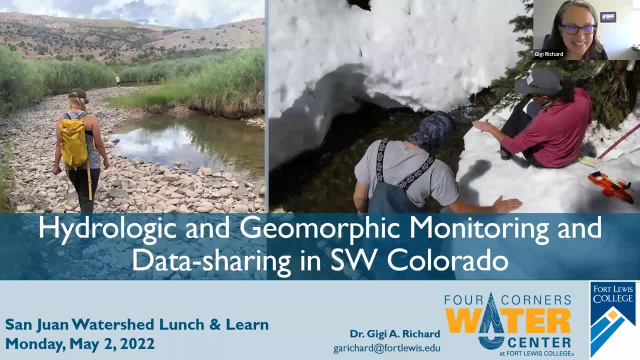 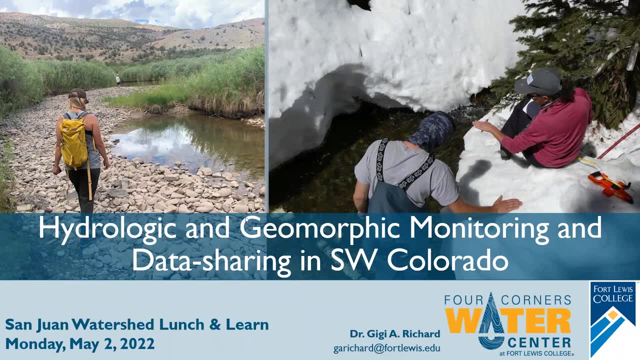 Okay. Okay, there we go. Are you seeing my screen? Yes, We can see your screen. We can hear you, Okay. Well, hopefully that'll be the last time that happens. All right, I'm not sure where I where I got cut off, but I'll be sharing about a. 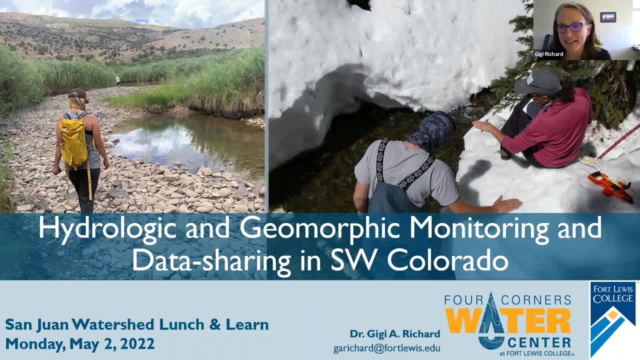 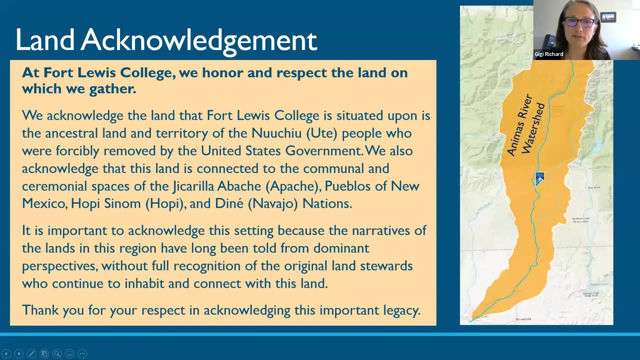 geomorphic monitoring effort on the Dolores and then some small watershed snowmelt hydrology work in the Animas watershed. that's part of a statewide effort, collaboration with CSU in Fort Collins. So before I get started I just want to do a land acknowledgement at Fort. 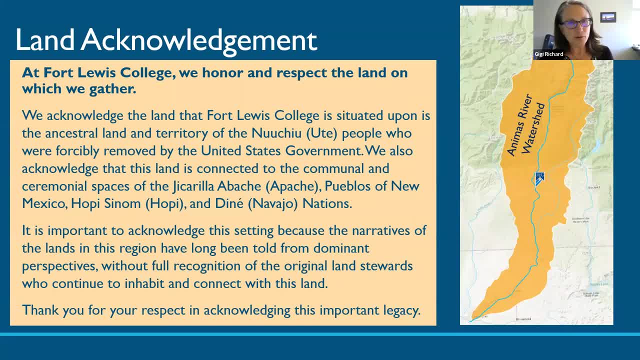 Lewis College. We always start every event, even virtual ones, with an acknowledgement of the land on which we gather, and Fort Lewis College is situated in the Animas River Watershed, which is the ancestral land of a number of indigenous tribes, including the Ute, the Hickory Apache. 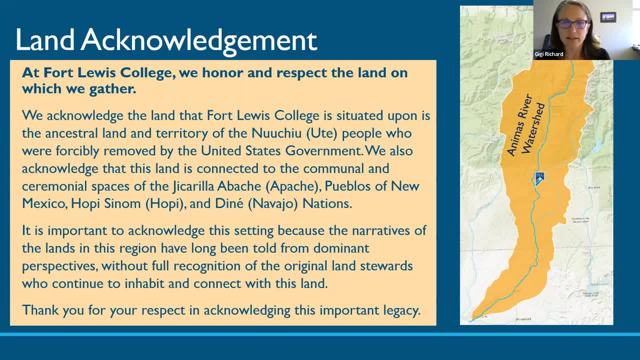 the Pueblos of New Mexico, the Hopi and the Diné Nations, And we acknowledge the setting because the narratives of the land in this region have long been told from a dominant perspective, Without full recognition of the stewards who continue to inhabit and connect with this land. 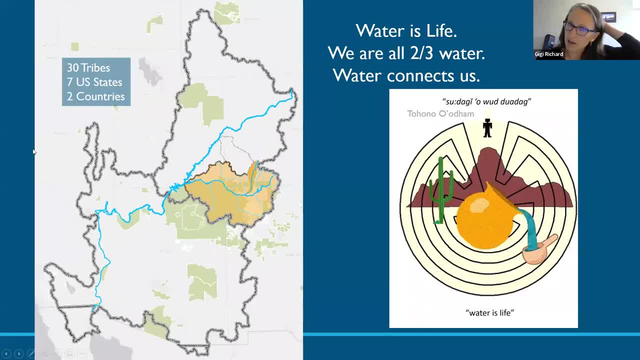 And from the water center's perspective, we also always want to acknowledge that we are all two thirds water, and water connects us all- and that we are part of a much larger watershed, And what we do here in the headwaters flows downstream to our downstream neighbors. 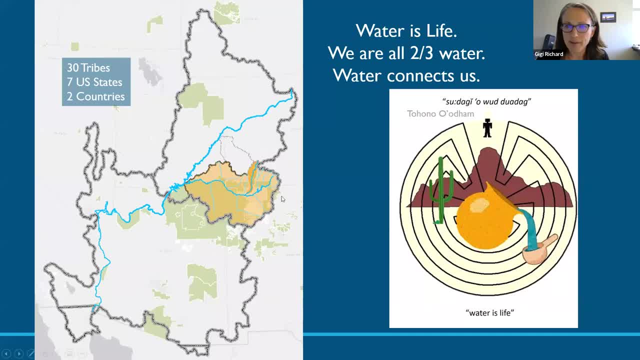 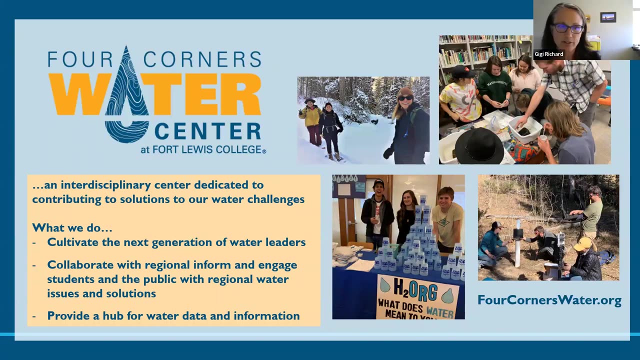 So we try to keep that in mind As well, Um, and I just wanted to point out- you know I'll be talking about the Animas Watershed and then the Dolores as well, which is outlined in gray here. Um, before I get into those two projects, I wanted to share a little bit about the water center at Fort. 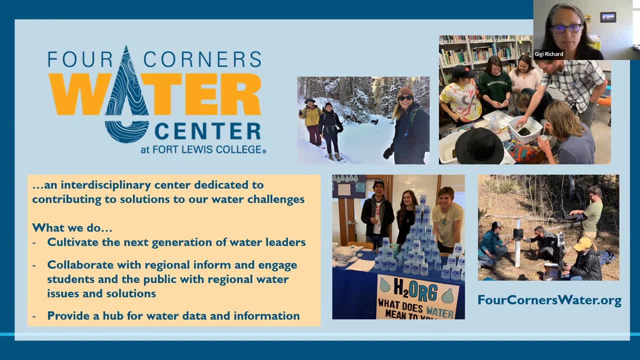 Lewis. It was started in 2019,, uh, by President Tom Striticus, Um, and we are an interdisciplinary center dedicated to working towards solutions to our water challenges And Okay, Okay, Okay, Okay. So we've been working for a long time. 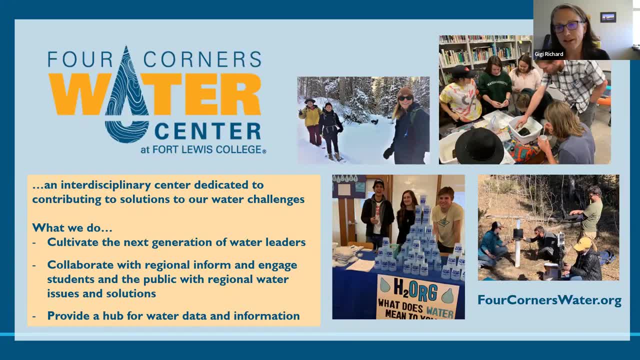 Um, and we've been working for a long time, Um, and we've been working for a long time, And we've been working for a long time And we've been working for a long time. Um, and in order to do that, what we're working on is, um, cultivating that next generation of water leaders. 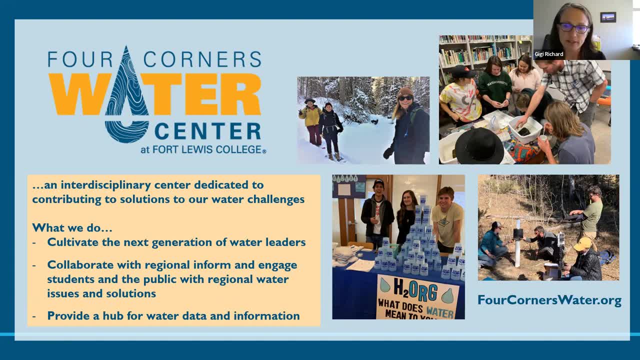 So trying to get our students engaged with local water issues, Um and research and studies. Fort Lewis has a really amazing breadth Of faculty who are working on water issues, And so we're working to create some water curriculum that take advantage of all of that amazing strength that we have across disciplines on campus. 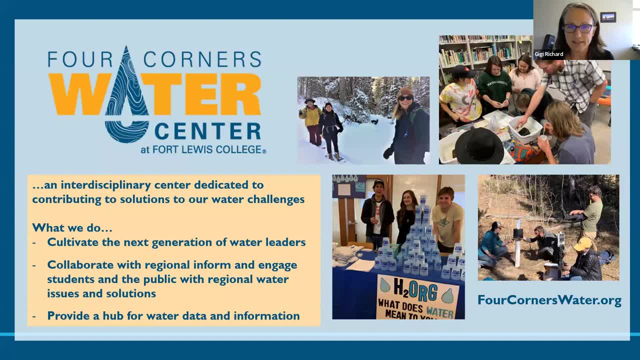 Um, and then I'll also talk a little bit about what we're doing with this infrastructure And um, but I think- according to somebody that has a broad Um, but I think can potentially be a great resource for the region. Um, if you're interested in learning more about the Water Center, our website is fourcornerswaterorg. 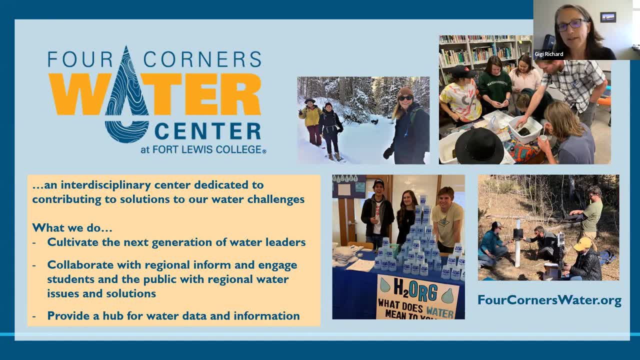 And on that website, if you scroll to the bottom, you can find our social media feeds and then also sign up for our newsletter, Um. we only send two newsletters a month and what we try to do is provide a um, a truly accessible and effluent set of people with pretty coming out of water facilities. 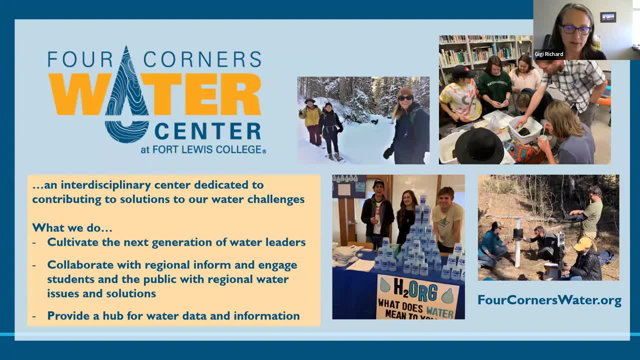 Um, um, They may be looking elsewhere- compendium of events and webinars of relevance to Four Corners: regional water, So basically the Dolores and San Juan River watersheds, And then we also share some Colorado statewide water news and events too. Also there's a focus to some extent for student jobs, internships. 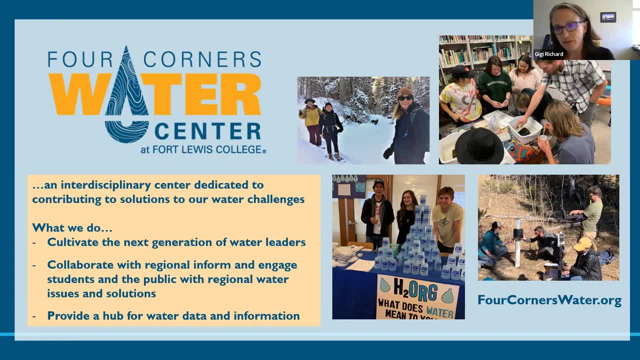 that sort of thing. So one of the things that we do is host a happy hour monthly for water professionals. It's usually on the third or fourth Wednesday of the month at 5 pm in Durango. So you can find out more about that on our website as well. So if anyone has questions about the 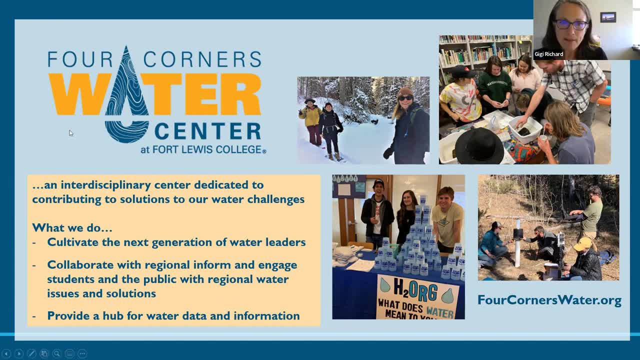 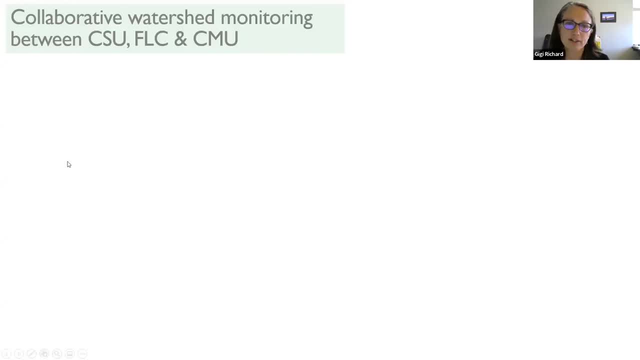 Water Center, don't hesitate to reach out. So I'm going to start off talking about our watershed model. So this is a collaborative effort that's been ongoing since 2015 between Colorado State University and Fort Collins, Fort Lewis College and Colorado Mesa in Grand Junction. So there 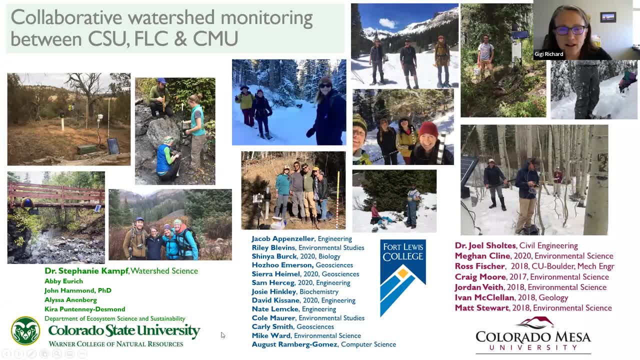 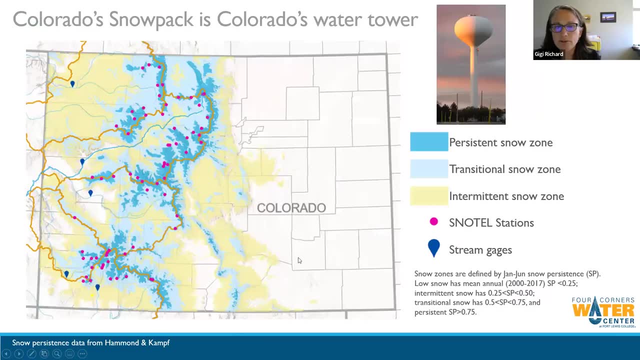 have been numerous students and faculty at all of these institutions involved in this effort And it's been a really neat opportunity to get undergraduates engaged in some hydrologic monitoring and research. So the idea for this project came from Dr Stephanie Camp. She's really the lead for this project. She's 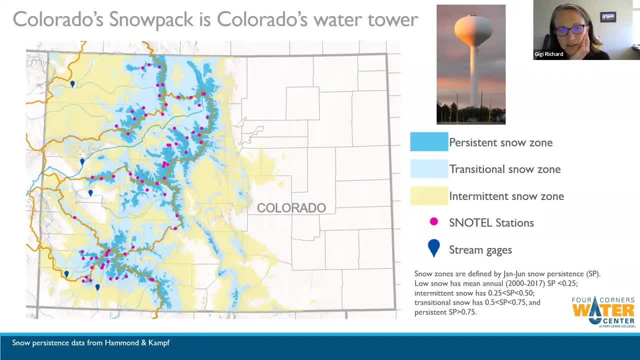 in watershed science at CSU in Fort Collins And she had a graduate student, John Hammond, who now has his PhD and works for USGS in Maryland. But as part of his PhD work he took MODIS satellite imagery and mapped throughout the entire West the persistence of snowpack. 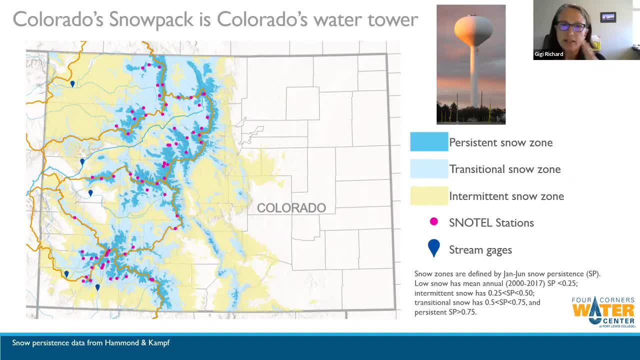 And classified each pixel as whether there was snow on in the pixel or snow off from January to June from the year 2000 through 2017.. If a pixel has snow on for more than 75% of the time from January to June, that pixel is classified as being in the persistent snow zone. 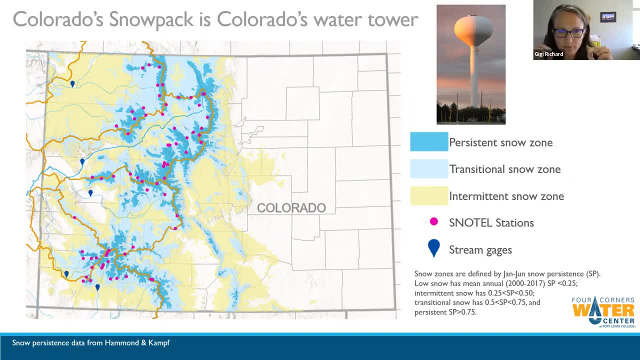 And so So persistent is snow on more than 75% of the time from January to June. Transitional is 50% to 75% of the time there's snow, And intermittent is 25 to 50% of the time there's snow. 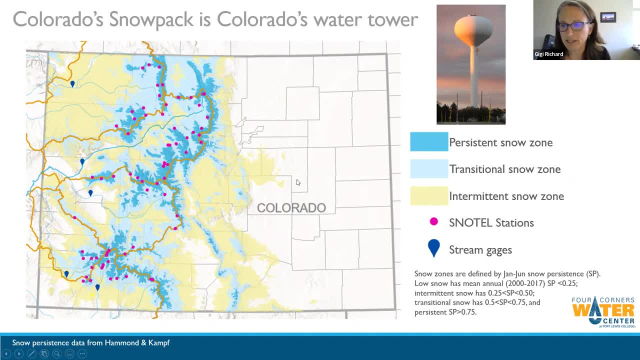 And then low snow, which in this map is shown with no shading, are areas where there's less than 25% of the time from January to June there's snow. So So you know one of the things that we know with our snowtel measurement- and of course, snow is- is extremely important for our water in Colorado, our snowpack is really our water tower. 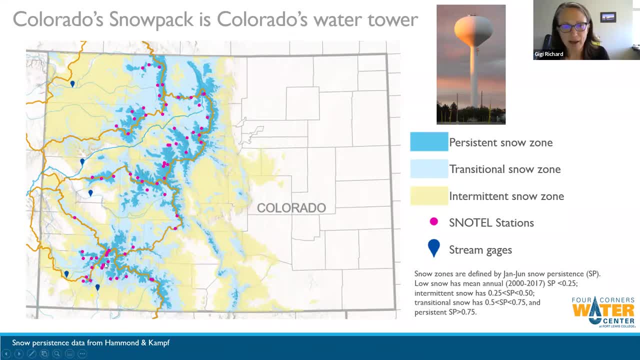 And so understanding the amount of water in our snowpack is really important for understanding what we're, what's going to happen with our runoff and our stream flow, And in Colorado, our snowtel measuring sites, which are run by the, by NRCS, are primarily a. 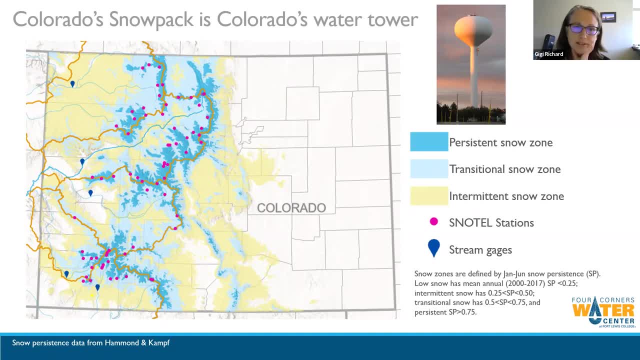 really up in that persistent snow zone. So we don't measure our transitional or intermittent snow zones as frequently spatially. So one of the efforts with this project is to try to better understand what's going on with our watershed hydrology in those three snow. 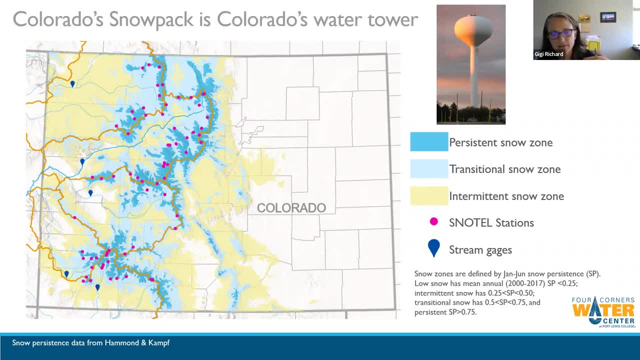 zones, from persistent through transitional, down to intermittent, in different regions of the state And to also, you know, we understand too that our intermittent snow zone, we know, is much more vulnerable as climate changes, as climate warms, So understanding what's going on with that more vulnerable intermittent snow zone and even into the transitional snow. 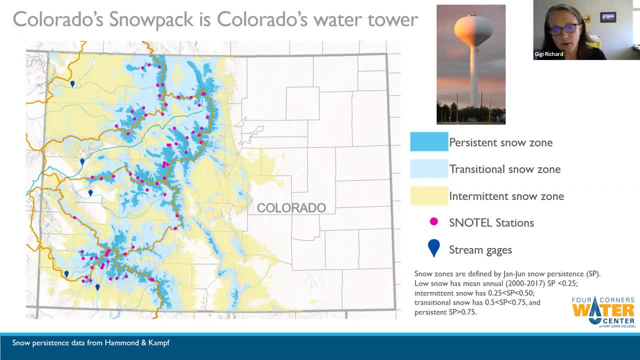 zone Can be really valuable for our water resource managers as we move into a warming climate. You know another thing we might notice with our monitoring and this: this map only shows five stream gauges because I pulled this from a different analysis that we did, but 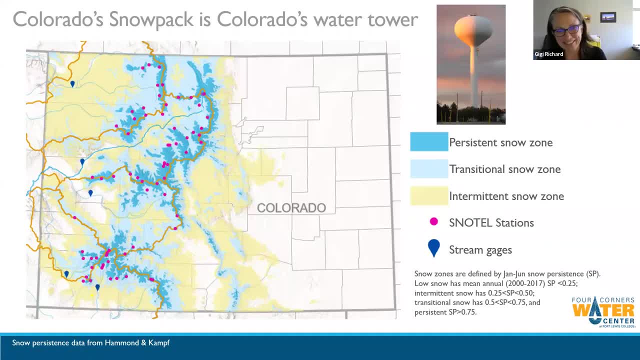 generally, we tend to measure streamflow lower down in our watershed. so we're measuring snow really high and streamflow lower down, And so one of the other efforts here is to have a little bit of data To better look at how streamflow is generated in these small watersheds. 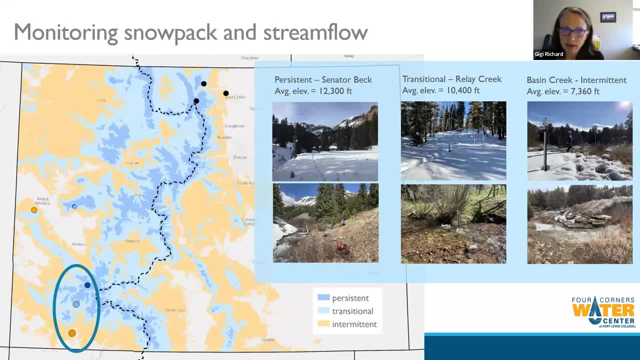 So there are 12 monitoring stations around the state. Well, actually I should say there were 12 monitoring stations around the state. The ones that were supported by CMU have now been removed, But Stephanie still supports some in the in the front range above Fort Collins and 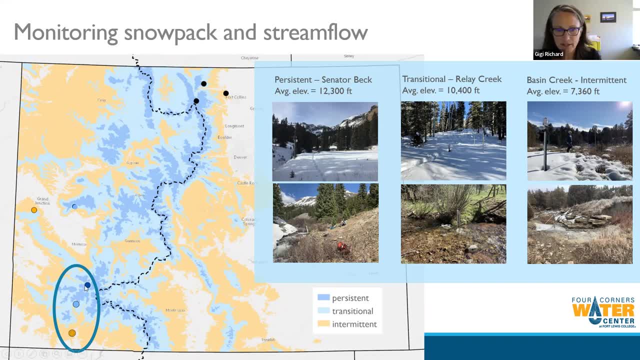 these are our three sites In the Animas River watershed. our persistent snow zone site is Senator Beck Basin, which is technically actually just outside of the Animas River watershed. it's at the very top of Red Mountain Pass and it is. it does flow into the Yoncum Pagre, but it is right at the 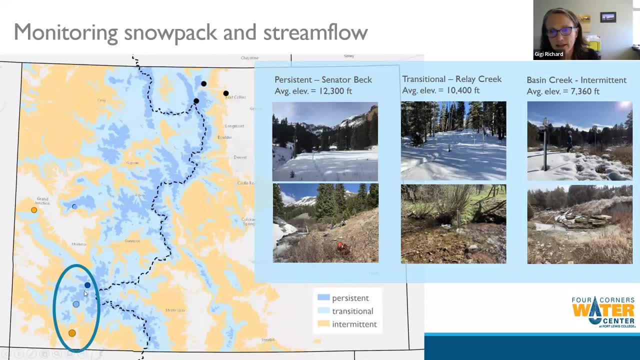 top. We chose that site because it is a long term, a site that's been monitored long term by the Center for Snow and Avalanche Studies, So there's a lot of information, There's a lot of valuable data there, and we actually share data with them and they. 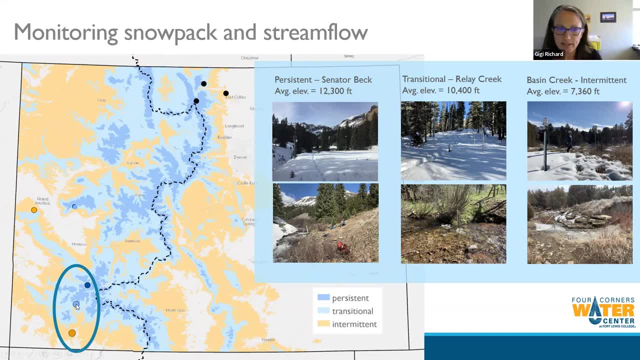 share their data with us. so our transitional site is at Relay Creek, which is in the upper Hermosa watershed. it's above the area that burned in the 416 fire and it's kind of behind Purgatory Ski Resort. And then our intermittent site is down at Basin Creek, which is a creek that flows into. 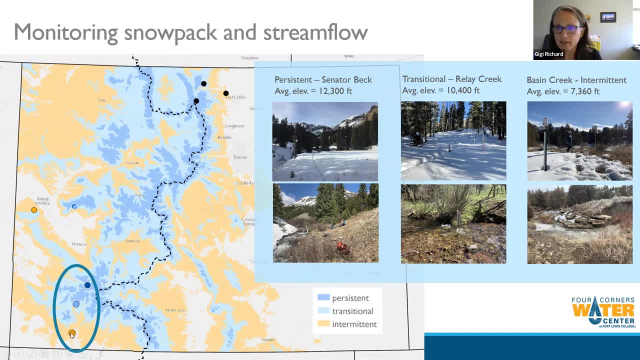 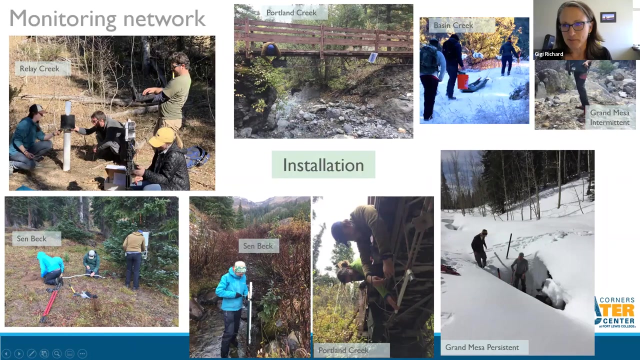 Lake Nighthorse And we partner with The Bureau of Reclamation and the Animas La Plata Operations, Maintenance and Replacement Organization for operating that site. So those are our three monitoring stations in the Animas River watershed. So what's involved in this network- and this is some of this is just a little bit of fun. 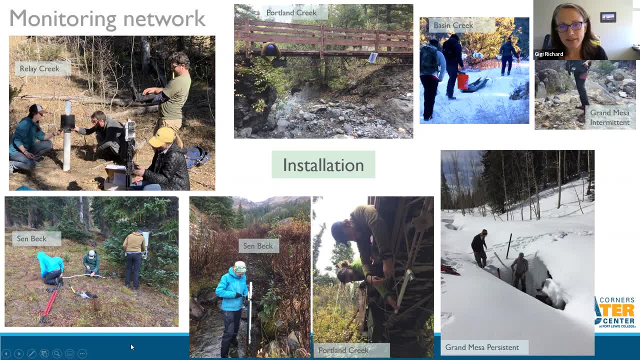 sort of sharing what we've done with students. the installation at all these sites is always can often be really challenging. it's been amazing how difficult it is to find small watersheds that are entirely in one of these snow persistent zones that are not regulated. 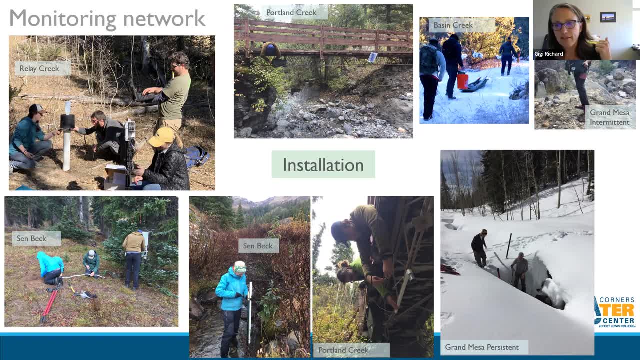 by any kind of diversion or dam or structure that don't have a lot of roads or other disturbance in the watershed and that we can access year round. so wintertime access can be challenging and problematic But it's. It's been a fun effort to get these this setup. 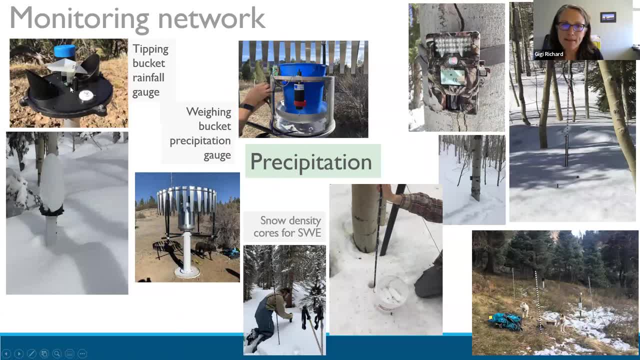 So at each of these stations we have either a tipping bucket or weighing bucket rain gauge. We have wildlife cameras pointed at snow stakes to measure snow depth. We, every time we visit, we'll take cores to get snow density so we can get our snow water. 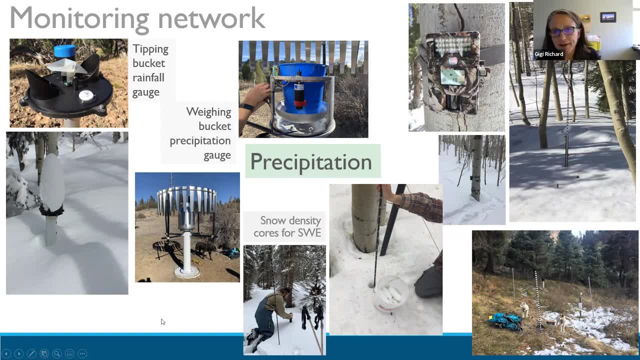 equivalent. So measuring precipitation and all of these methods are not without challenges. tipping bucket rain gauges don't do well when it freezes The wildlife cameras. I'll share some interesting pictures with you, but we've had a lot of problems with those. 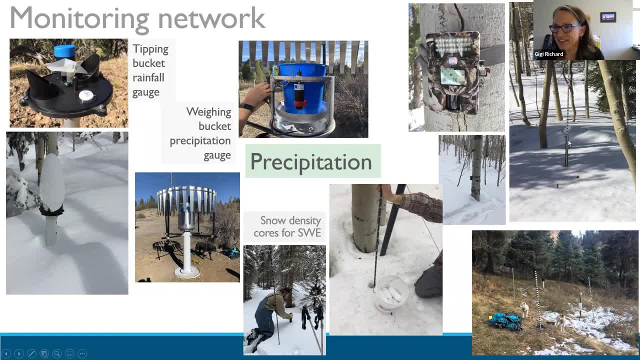 Oh, and I should mention too, I have a student right now who's working on using machine learning to process the images from these and detect the snow stakes and and automate them. So I'm going to share a picture of her Measuring of snow depth from the stakes. 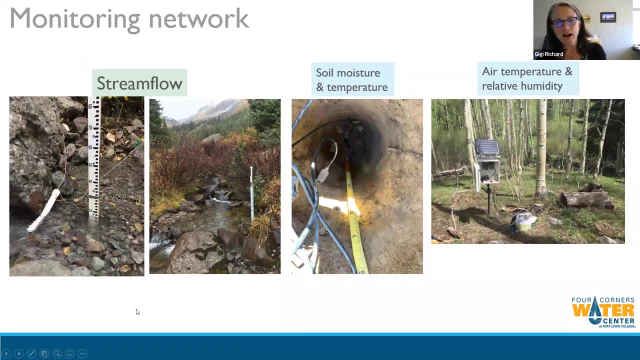 So another sort of exciting sideline to this, We also measure streamflow at each of the sites. some of the sites have pressure transducers and some have capacitance rods for measuring depth. and then we do discharge measurements whenever we go visit to develop a rating curve so we can estimate or measure discharge. 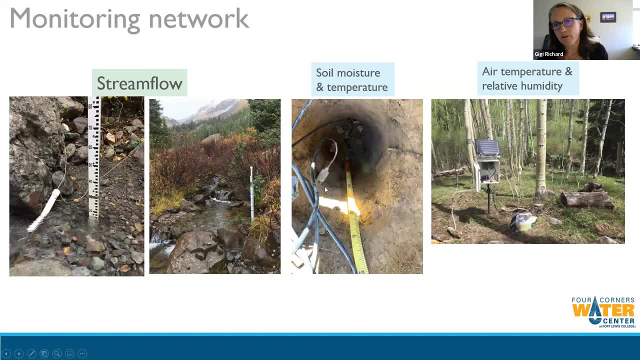 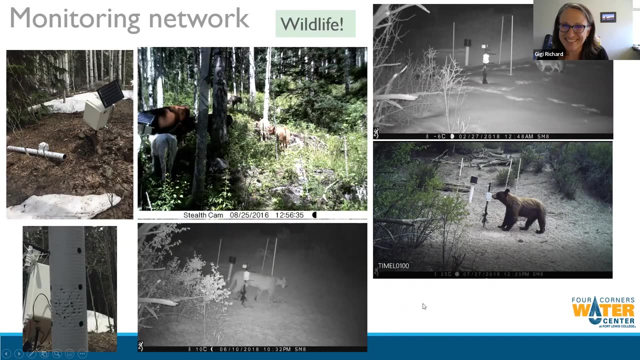 At each site. we also measure soil moisture and temperature. So we have soil moisture and temperature, We have soil moisture sensors at three depths, And then we also measure air temp and, at some sites, relative humidity. We also sometimes monitor wildlife and have challenges with animals. one of the sites 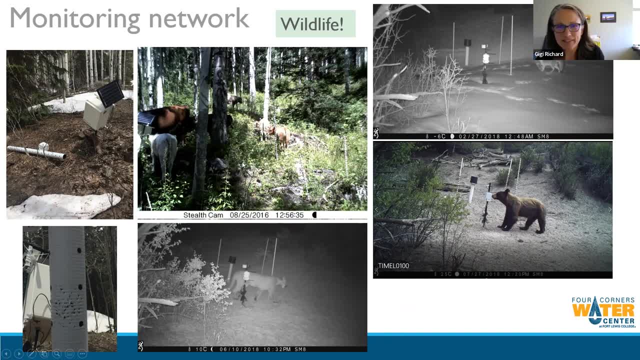 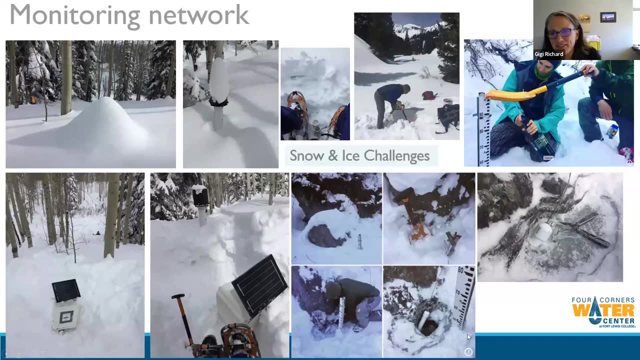 on the Grand Mesa. there was a grazing permit there and the cows would move through, and and then we have have some fun going through the images from the wildlife cameras each time We pick them up to see Who else visited our sites. We also often have a lot of challenges with exactly the thing that we're measuring and 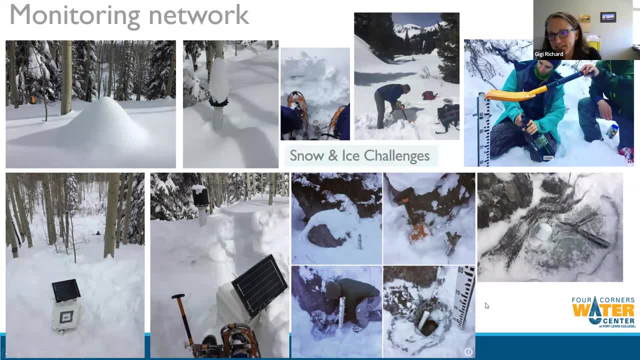 that is snow and water. Digging these sites out and the freezing that can happen and that sometimes breaks things can be really challenging. It's a really ingenious MacGyver students to try to get this PT out of the ice they had brought. 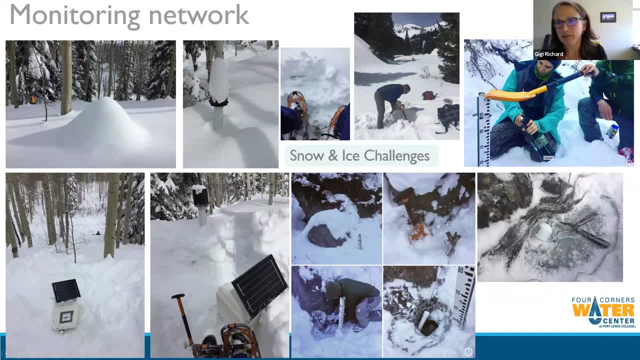 A propane torch but realize we didn't want to melt the plastic and so they put water in the snow shovel and heated up the snow shovel to get the water hot and then poured it in there and and I got- we got PT out. so that was a clever solution. 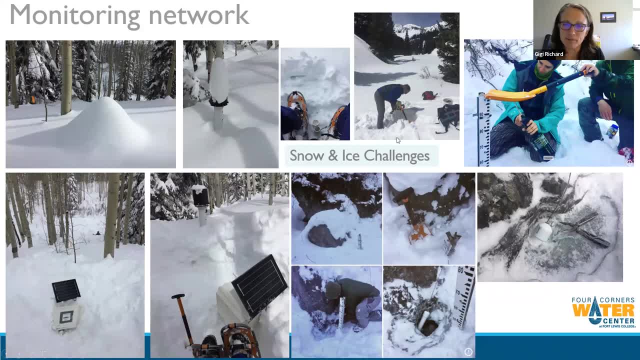 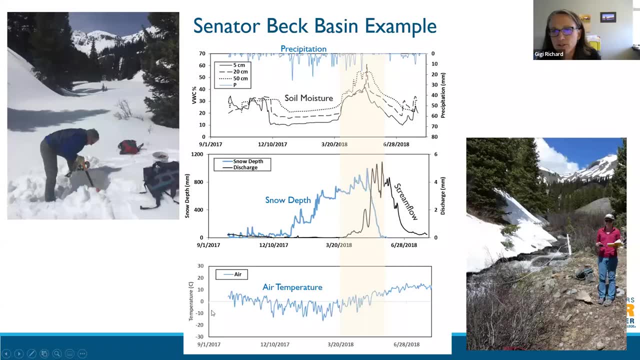 Sometimes we can't find the stream gauges because they're completely buried. that that's been a challenge. That was especially a challenge in 2019 of the tenant. So to give you an idea of some of the data that we get from these, 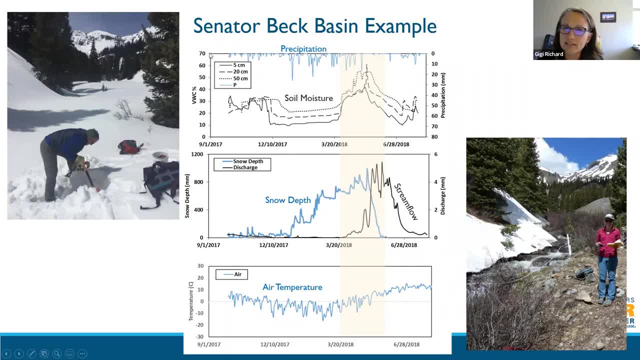 And I know this is kind of busy, but I'll step through it. This is that, Senator, back, Looking at the 2018 water year, This is the first year that we monitored up there, This top one up top up here we have precipitation coming down from the top using this axis. 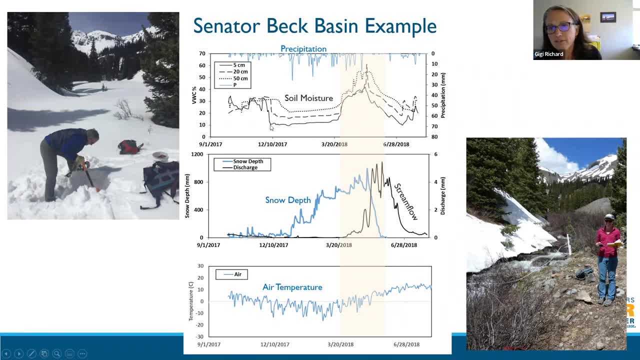 here We have soil moisture at five centimeters with the solid line, 20 centimeters with the big dash line and 50 centimeters With the dotted line. accumulation of snow depth- I don't have sweet plotted on this one- and then stream flow is discharged in millimeters. 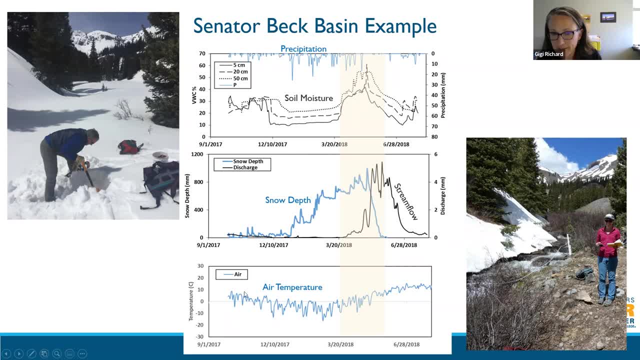 per day over the watershed. And and then air temperature, And so we can see our accumulation of snow as air temperatures start to warm up and our days start to get longer. The response: The first thing that happens when the snow starts to melt. 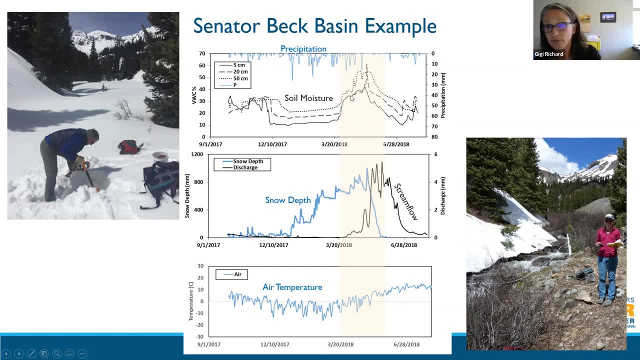 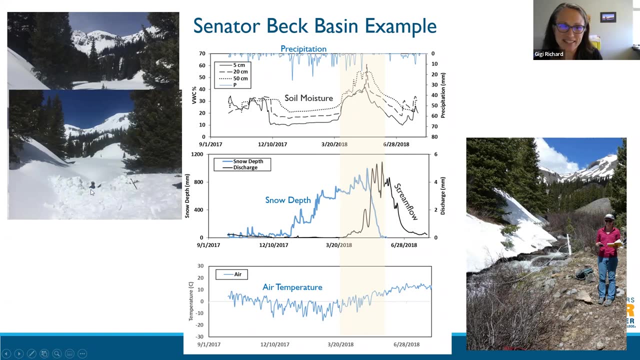 Is it soaks into the ground? we see our soil moisture responding and then, following that, we see stream flow response. So, oh, I mentioned that we couldn't find our stream gauge here. we never did find it until the snow started to melt there, and when it did emerge, this was 2019- it was broken. 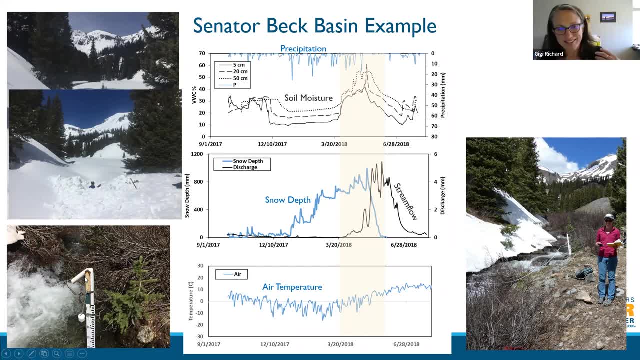 And so, of course, the year that we most wanted to see the response, because this is one of our bigger problems. And so, you know, in the winter water years, recent years, The instrumentation was completely broken and we didn't get any stream flow data and 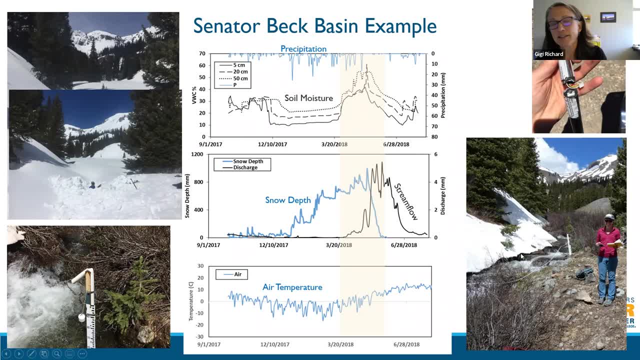 because of the depth of the flow, burying our depths of the snow, burying our solar panels. we also lost all of our soil moisture data that year, so really frustrating. Okay. so what are some of the things we've learned from this? oh, and I should have pointed: 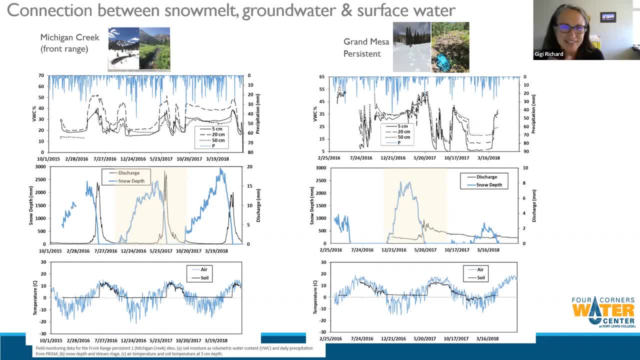 out that I'm not going to share a ton of really groundbreaking results because we're still have a lot of work to do on on all these data. one of the other things that we've learned is that having data collected by three institutions at 12 sites produces a lot of data and takes 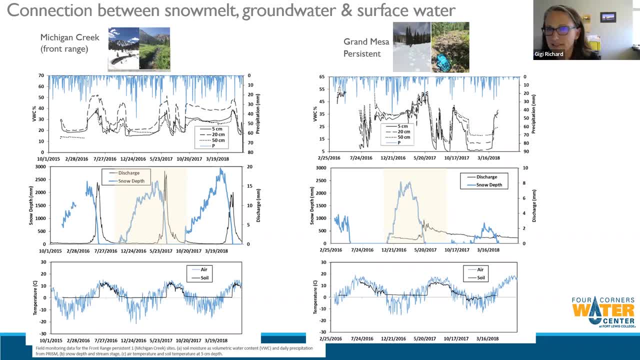 a lot of processing, a lot of challenges for data management, so it's been a good learning. So just interesting, you know, connection between snowmelt, groundwater and surface water are persistent site on the front range at Michigan Creek. So if you look at the snow depth here in blue- and I'm just going to focus right here on this 2017 water year- compared with the Grand Mesa, they had really similar snowpack, but check out the response in the stream. so really flashy, peaky hydrograph, whereas on 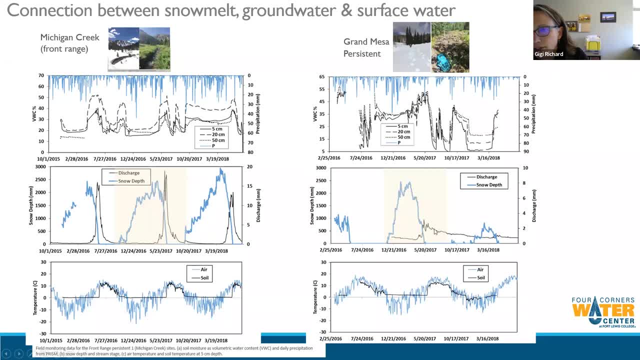 the Grand Mesa: high base flow and much lower runoff. and then our peak runoff: So much lower runoff, So much lower runoff, more attenuated snowmelt hydrograph with much higher base flow, which makes a lot of sense given the underlying geology of the Grand Mesa and how important groundwater and springs are. 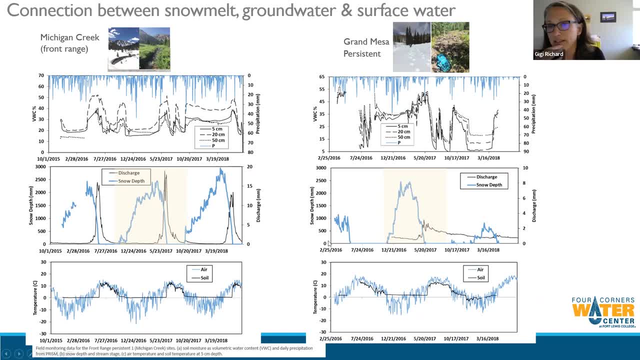 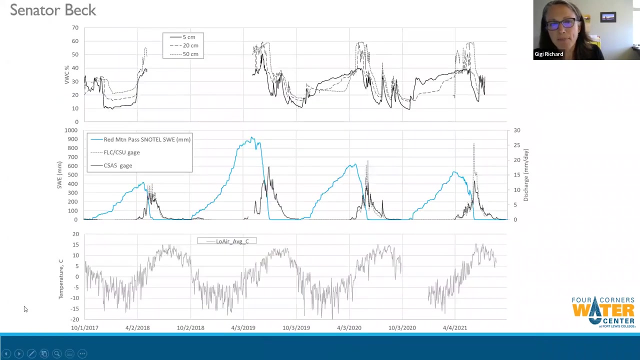 on the Grand Mesa, So something we really didn't expect. Another interesting thing: our original intermittent site on the Grand Mesa had no, the stream never flowed, And so it's helped us see and emphasize the importance of some other factors that we kind of weren't expecting through this process. So finally, just a few. 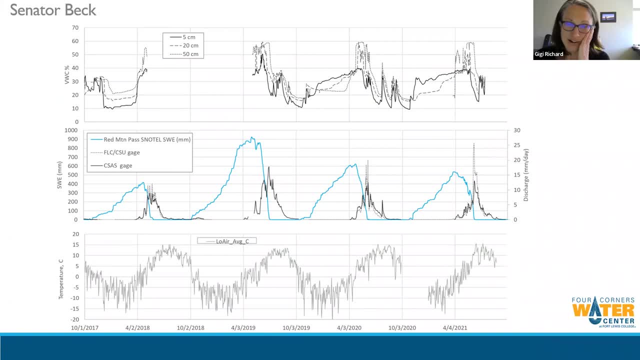 graphs showing our full record for our Animas station. So here is our Senator Beck. So this is our persistent snowpack station at the top of Red Mountain Pass, Similar to what we had before. here's our soil moisture. This is our big data gap. 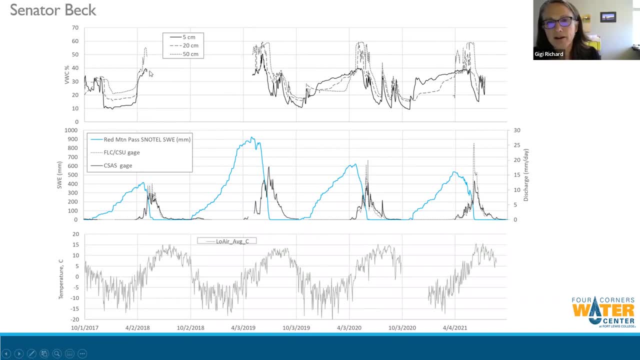 In that 2019 water year where our data logger there died. And then I've got the Red Mountain Pass snow tail, snow water equivalent 2018, recent drought year, 2019, much higher water year, And then our kind of more average snow years of 2020 and 2021.. And then the stream response measured. 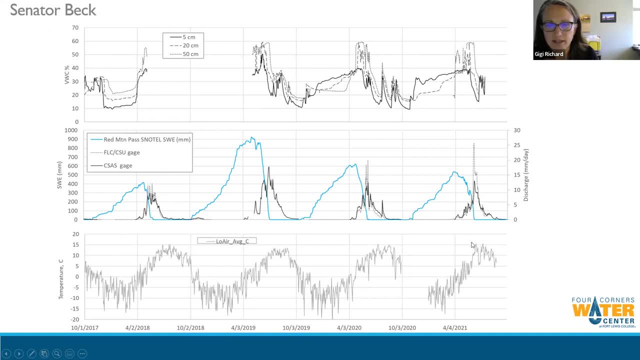 up to about 2,000 kilometers of discharge per day. So this is taking the rate of flow and spreading it out over the watershed And then our air temperature down here. So we can see as temperatures start to warm up and the snow starts to melt, our soil moisture starts to go up first and then. 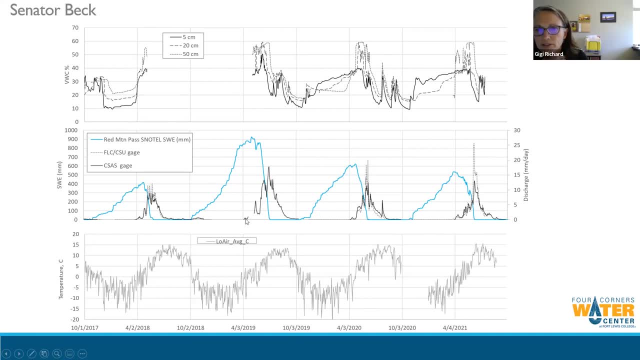 the stream flow begins to increase once we start to charge up the stream, And then the moisture in the soils, And I don't have any of our 2022 water year data. Okay, So then moving on. So Senator Beck is our longest data record for the Animas watershed. 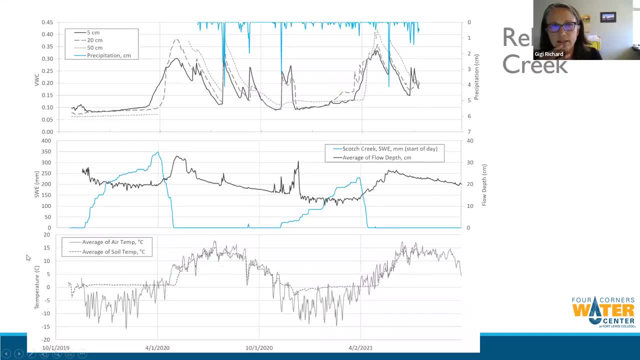 We installed that one in fall of 2017.. Moving down to our intermittent, or sorry, transitional site at Relay Creek, This is the one above Purgatory Snow water equivalent at the Scotch Creek. This is one of the sites where we had a lot of problems with the camera for our snow depth. 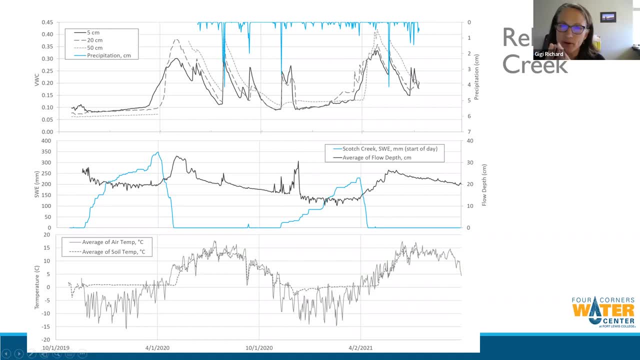 The good news is that for the time periods where we do have our snow depth data, the data match really closely with the Scotch Creek's no-till site, So we feel good about using the nearby snow-tel site for this watershed. Let's see So much lower snow water equivalent than at the persistent site. 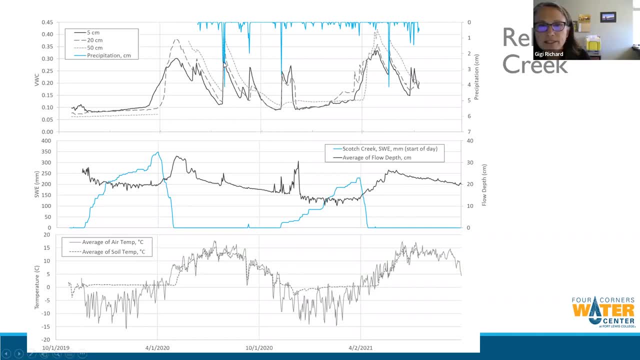 which is what we would expect. You can see really clear response of soil moisture to precipitation events. So each of these blue lines coming down is a precipitation event and we can see our soil moisture respond And moving down all the way down to the 50. 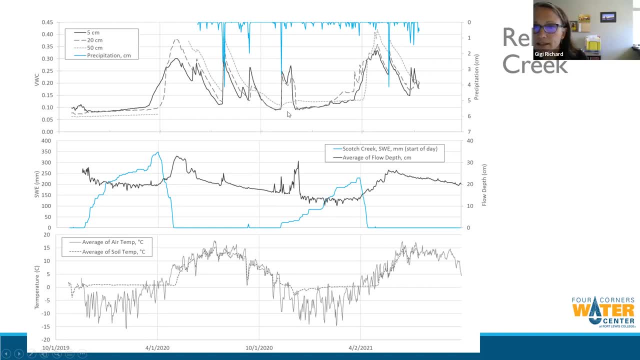 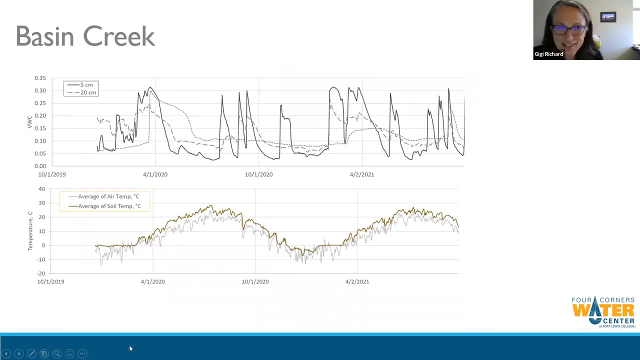 centimeter depth for some of these bigger precipitation events and the delayed stream flow response. So we see soil moisture coming up and then the stream flow with a little bit more delayed response And then our intermittent site has been really tricky At our intermittent. 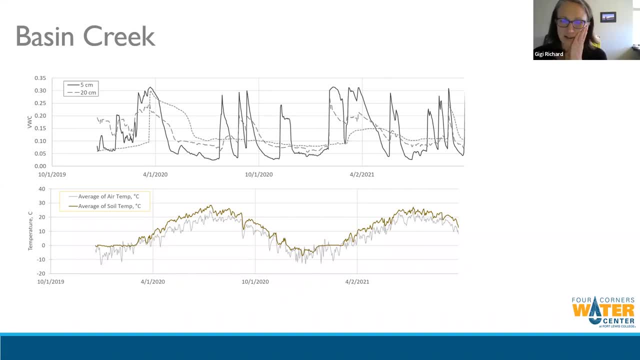 site, the stream. not surprisingly it's ephemeral. It's flashier and we've had a really hard time getting a decent rating curve for that site, so I don't actually have any of the flow depth to share with you. I've worked. 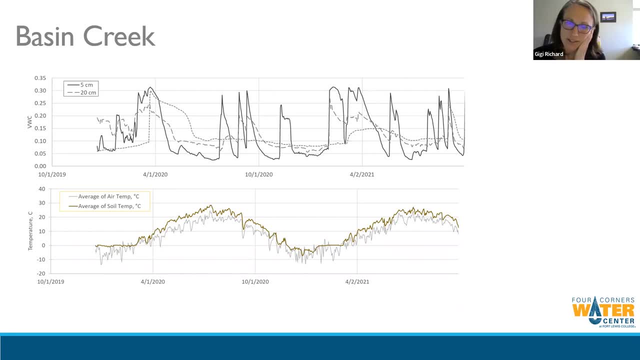 closely with Susan Beharie with the Bureau of Reclamation and she's actually done a lot more work on taking our flow depth data and trying to get some sort of useful stream flow data out of that. And, not surprisingly, with the intermittent snowpack we see a lot. 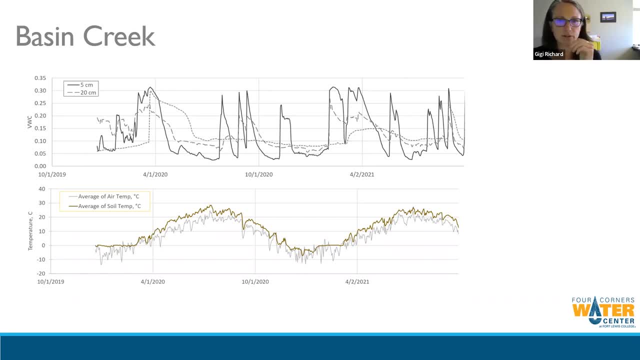 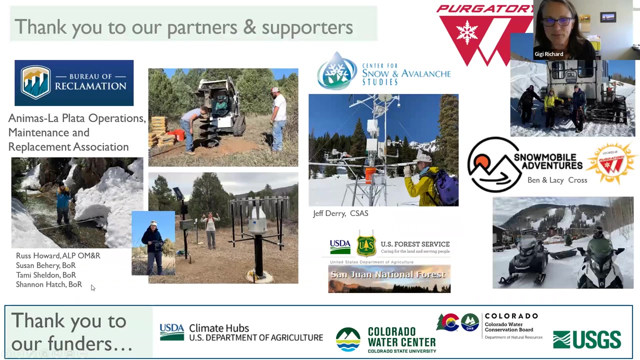 more spikes and peaks in soil moisture, a lot warmer soils too, and then a little bit more responsiveness in the soil moisture from the monsoonal peaks in the summer. So that's kind of an overview of where we're at with our monitoring, and I did want to point out 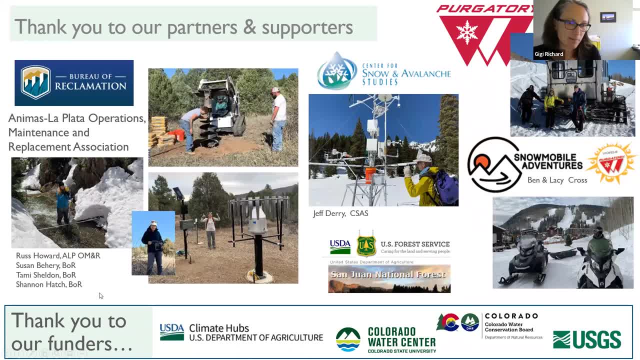 that this project is a big collaboration amongst a lot of our state agencies. We've done a lot of different entities and, without the support of the Bureau of Reclamation and ALP, O&M, the Center for Snow and Avalanche Studies, we've, you know, permits and working with the Forest. 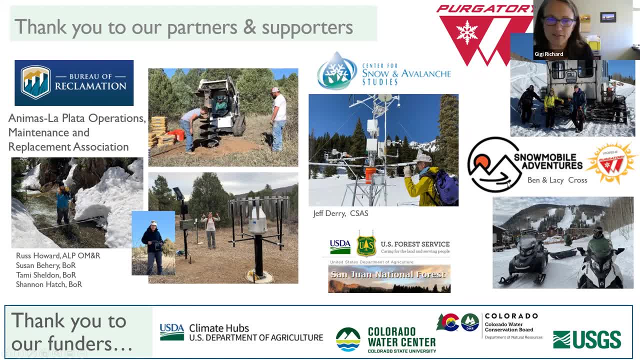 Service, and then Purgatory Resort and Snowmobile Adventures have helped us get back to our intermittent site. It would be quite a long ski in. And then we also have had funding from USDA ARS, Southwest Climate Hub, the Colorado Water Center, CWCB and USGS. So it's been 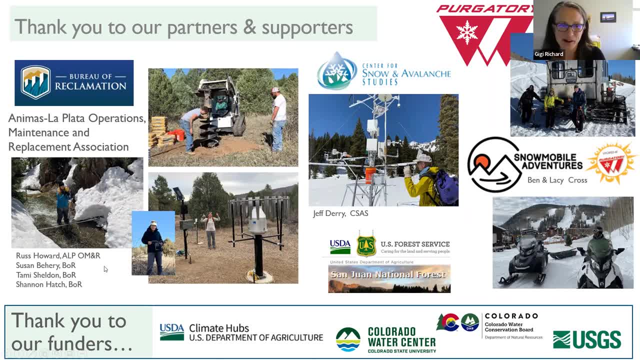 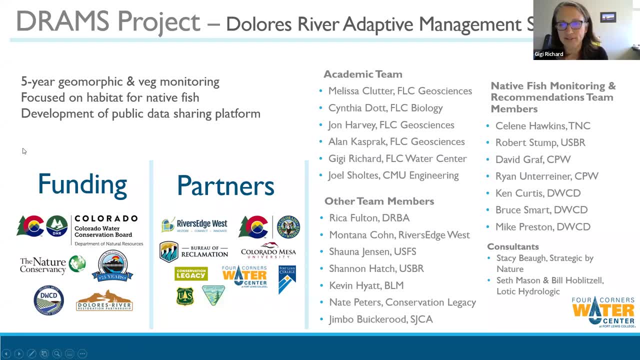 a very well-supported, collaborative, cooperative effort. Okay, now I'm going to shift gears and talk about this Dolores River geomorphic monitoring effort so that I can share a little bit about the database that we're working on associated with this project. So this project. 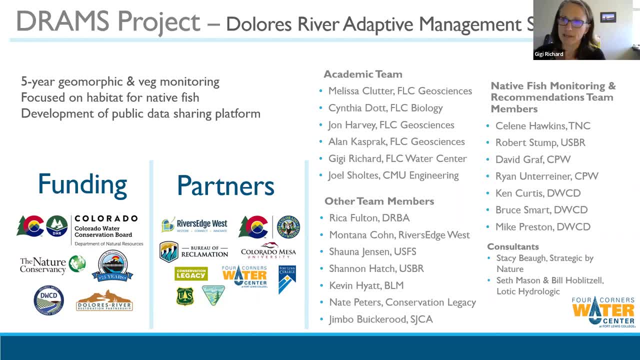 are actually. The acronym is DRAMS for the Dolores River Adaptive Management Support Project, And once again this is a big collaborative effort. The academic team includes geology and biology faculty at Fort Lewis and Joel Schultes, who's an engineering professor at CMU in Grand Junction. 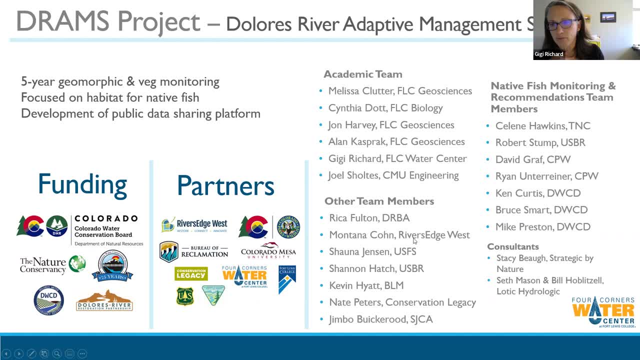 In addition, many other partners, including Rivers Edge West Bureau of Reclamation, Forest Service, BLM Conservation Legacy, San Juan Citizens and the Colorado Water Center. And then the project was initiated by questions that were raised by the Native Fish Monitoring and Recommendations team, which is a very large group of stakeholders in the 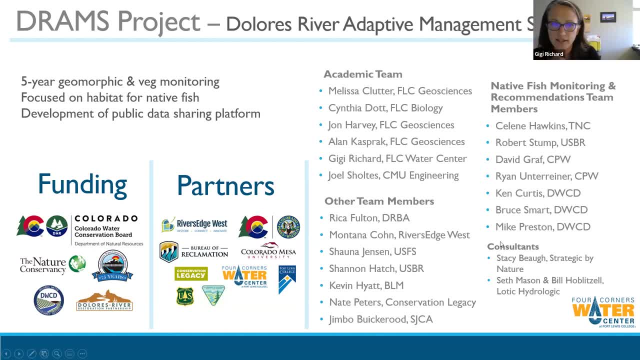 Dolores River Basin and a subset of them have been involved in our project. Our primary funding's from CWCB, but there's a lot of support from Dolores Water Conservancy District, Nature Conservancy, Southwestern Water Conservation District and Dolores River Restoration Partnership. So some of the funding is just great. This is the project and it is funded by a grant from the CWCB. There's a lot of funding that was funded by the CWCB, but the $3 million for Water Conservation District's. other projects in the community are on the GoTheard project and the project is funded by the. 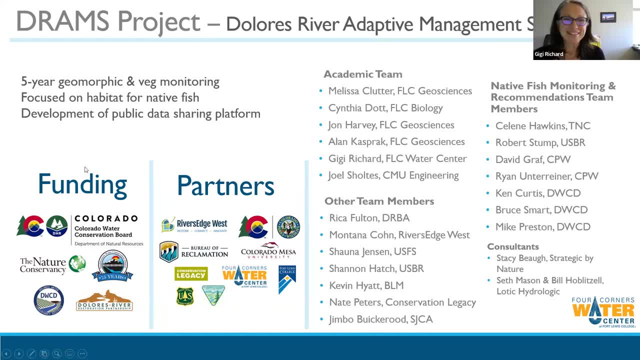 CWCB, our Northwest Water Conservation District, and the Northwest Water Conservation District and the and Dolores River Restoration Partnership. So it's a five-year monitoring effort We started last year. We spent about six months or so developing a monitoring protocol and the 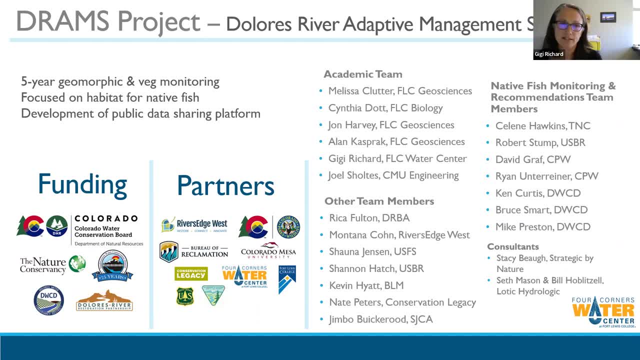 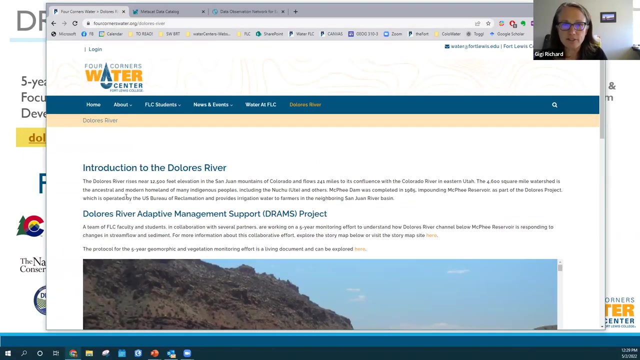 underlying motivation is focused on habitat for native fish- I'll talk a little bit more about that- and then it also includes development of public sharing data platform, And as part of this project, we have developed a website which I will share with you. If you go to DoloresRiverorg, it takes you to the site, and on the site we have a story map. 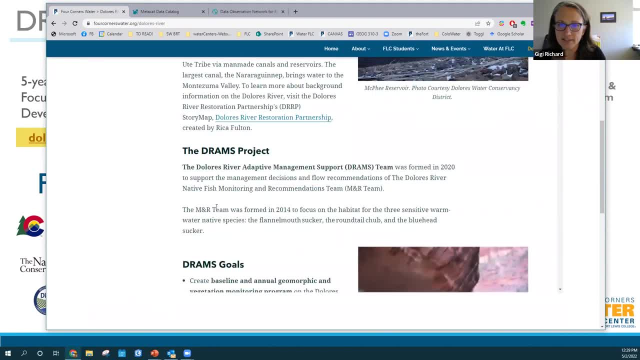 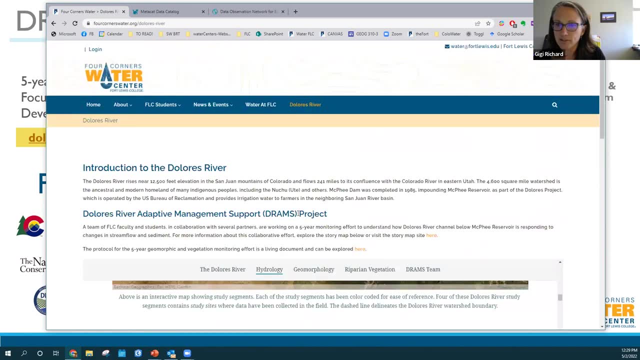 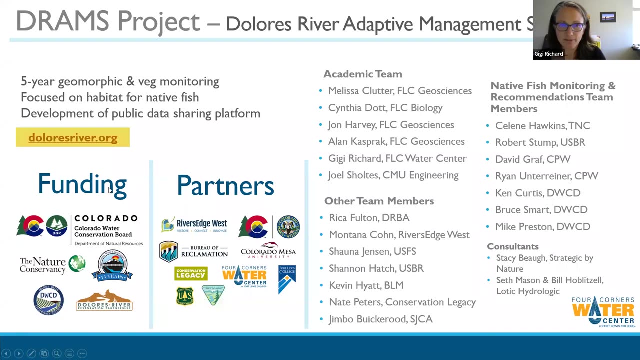 that tells the story of the DRAMS project, So this is a great place to go look, Yeah, At some of the work that we've been doing, and also you can access our monitoring protocol report here as well, So you can head over to DoloresRiverorg if you want to check that out. 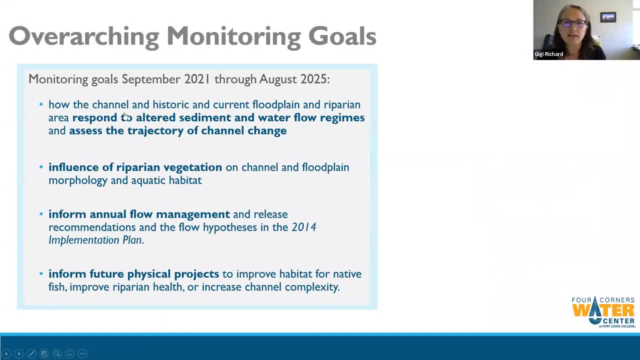 The goals of the monitoring effort are focused on how the channel and the floodplain and riparian area are responding to the new water and sediment regime following the closure of McPhee Dam and to attempt to assess the trajectory of channel change. We're very interested in what's going on with riparian vegetation, because that's been 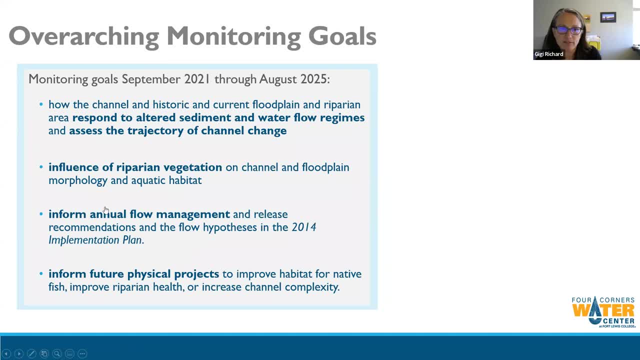 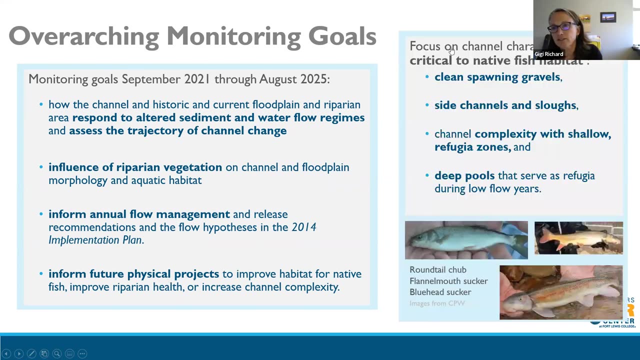 an important driver in what's happening with simplification of the channel. The idea is that these data could help inform flow management and release recommendations, and also potentially inform future physical projects for restoration. The focus on channel characteristics is on those that are critical to native fish habitat: The native fish. 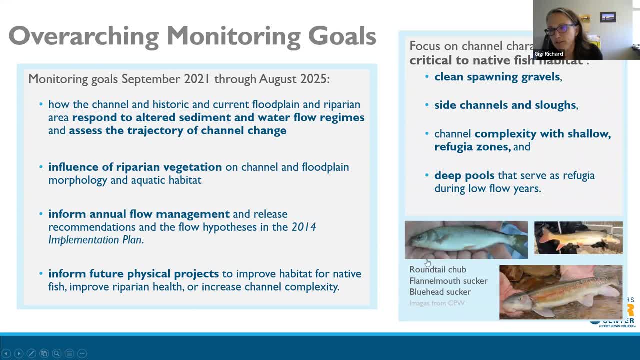 of interest are the three species of interest: the round-tailed chub, flint and mouse sucker and the bluehead sucker, And so looking at assessing clean spawning gravels, connection to side channels, channel complexity and pools. So that's kind of what we're looking at. 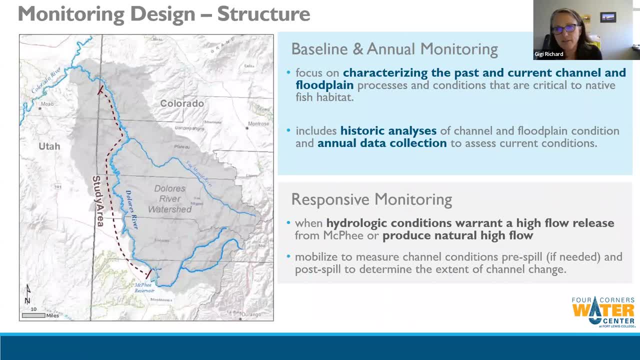 Our monitoring effort is divided into two main pieces. One is a set of monitoring that will happen every year, and then another effort is a responsive effort, and the idea is we want to be able to mobilize responsively when hydrologic conditions warrant a high flow release or if we're, and potentially also some of the 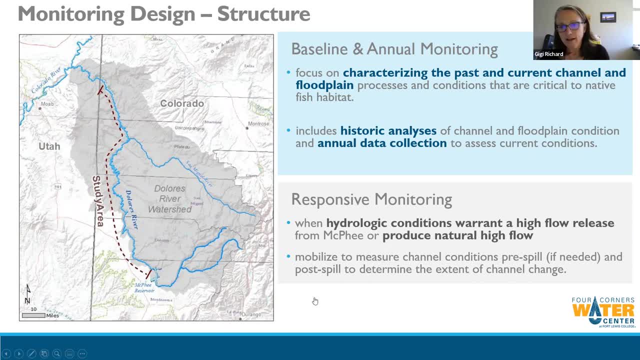 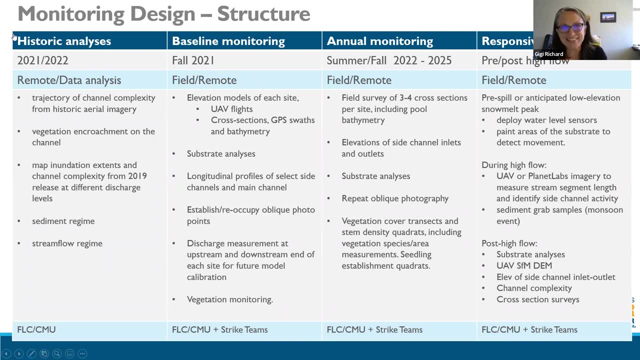 monsoonal flows, So we've seen some impact from that. So just, I know this is a lot of text on the slide but I just want to kind of share. like there's a lot happening associated with this monitoring, So a piece of it is historic analysis using remote sensing, and then historic 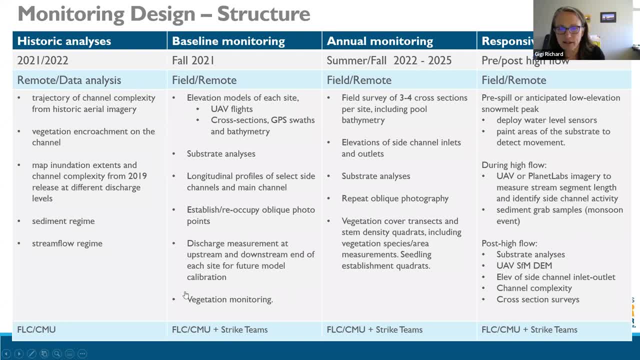 data. A piece of it was baseline monitoring that was accomplished last fall, including UAV flights, drone flights of our study sites- and I'll show you where those are in a sec- Some other topographic surveying, substrate analyses of the bedmovers and so on and so forth. So that's kind of what we're. 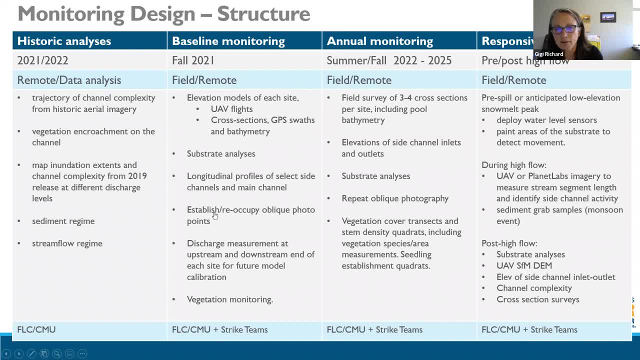 interested in learning is what we're seeing, how we're imagining what's going on. withushiwa and a couple of papers lunch. so weather material on profiles of side channels, oblique repeat photo points, some discharge measurements for use in future: model calibration and then vegetation. 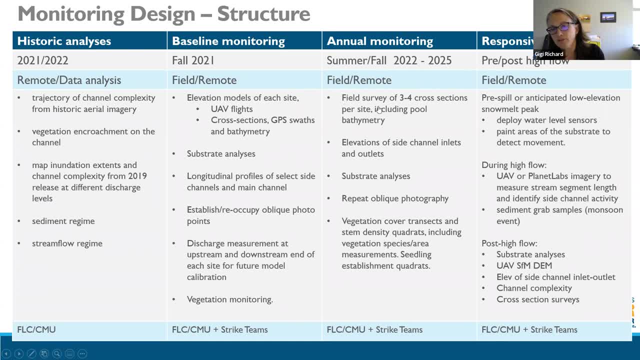 monitoring And then annually in the summer for veg data. in the fall for geomorph data, there will be some field surveys of cross sections, including pools, peat, oblique photography and then vegetative transects, and then, if we do have high flows, we will get out and deploy water level sensors, do some substrate movement detection efforts. 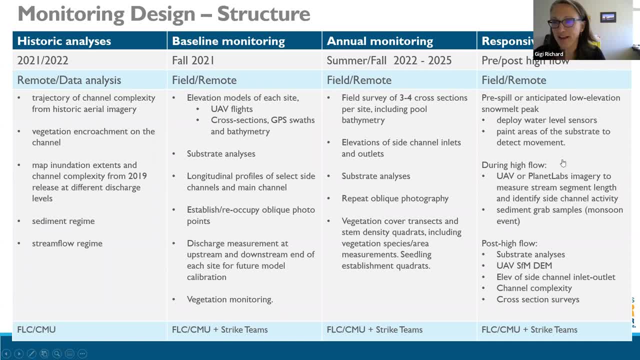 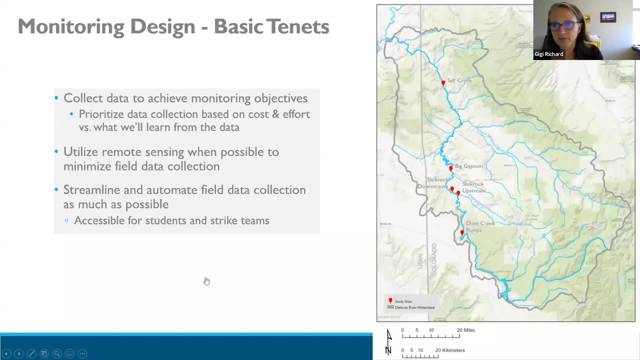 during the high flow, if possible they want to fly. do some drone flights and then, after high flow, definitely do a drone flight to see if there's any channel change and then redo some of the topographics for days. so it's a it's a pretty big effort. we have tried to streamline. 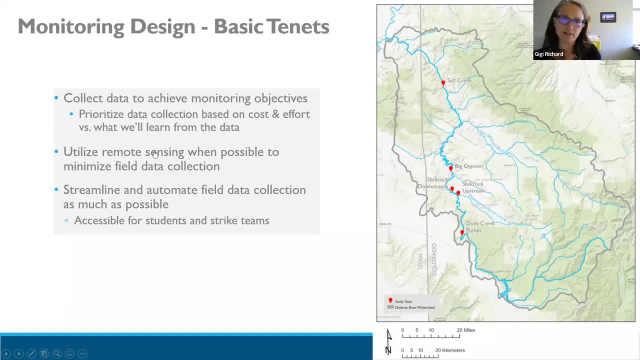 our monitoring so that we utilize remote sensing when possible to minimize field data collection, given the travel distances to the sites that can be make it hard to get out there, and we're also trying to focus on data that will support the monitoring. so the river has been broken into study segments, study reaches and field study sites. we have 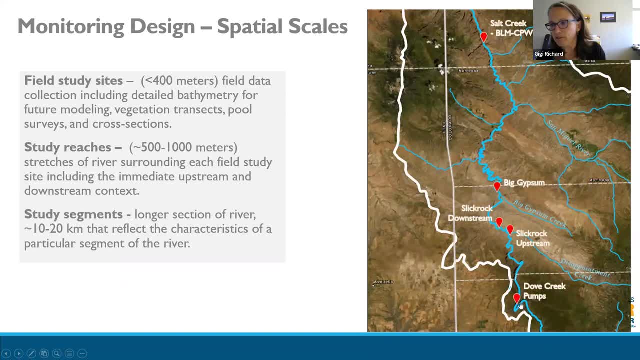 five field study sites from upstream to downstream: dove creek pumps that rock above and below this point of creek, one in big gypsum and one that below the confluence with the san miguel. the study segments are um is where they're doing a lot of remote sensing work. 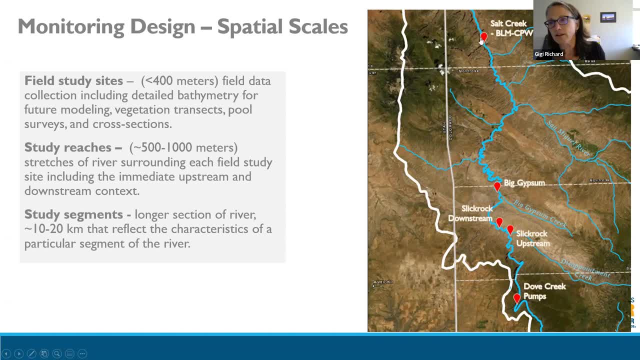 that i'll i'll share with you some results. the study reaches are where we're flying, doing the drone flights, and the field study sites are where we're actually doing on the ground, cross-section surveys. um, to give you a sense of just what these look like, dove creek pumps is up by the box, elder. 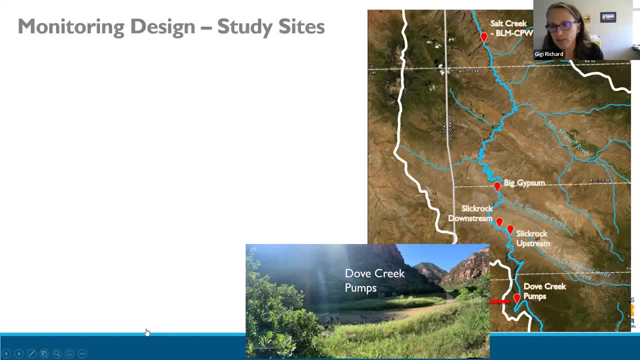 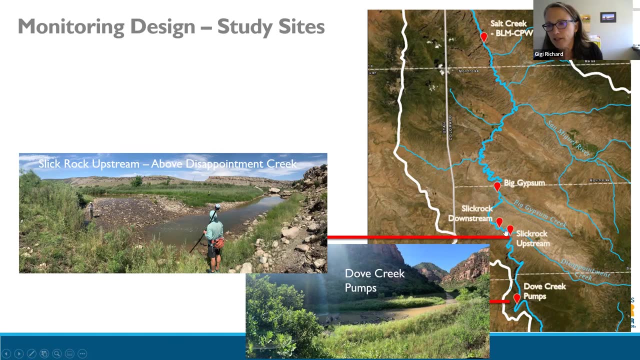 campground. it's a more. it's a more confined canyon. reach um disappointment creek brings in more sediment than water um so we see a change in the character of the river from above and below the disappointment creek. it's also key for fish, um changes in what's available for fish and also. 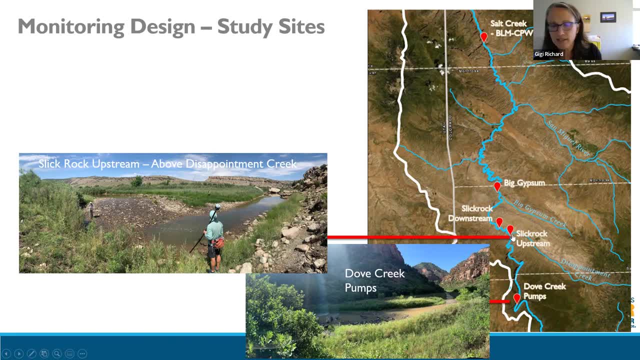 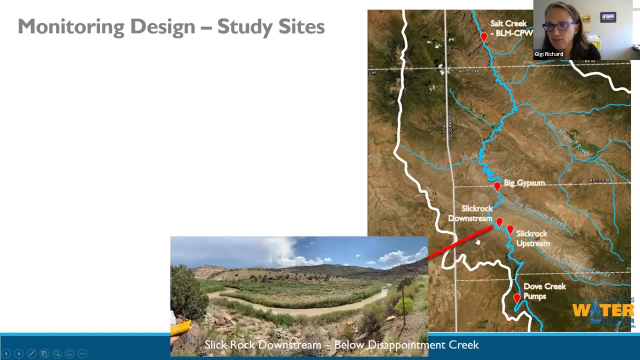 colorado parks and wildlife has a fish pit tag array at slick rock upstream. all of these three sites have been monitored in the past, um, over time, um, and let me jump ahead to now our slick rock downstream, so below disappointment creek, the big gypsum site has been monitored and we're 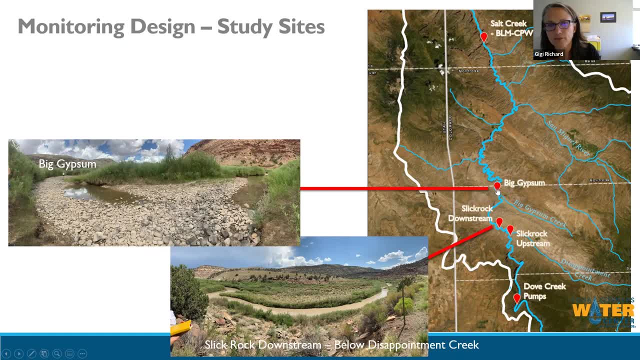 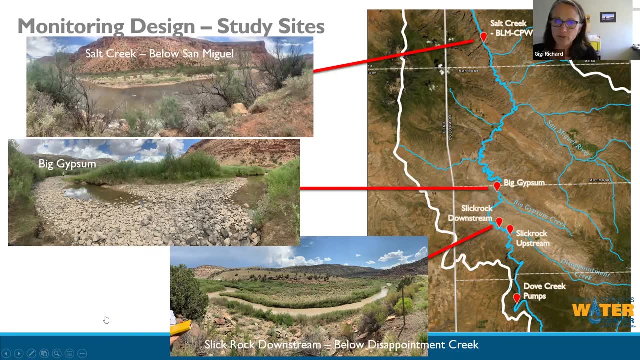 going to show you a little bit of the data that we had um for the next few slides, but it's also looking at what's going on on our bbc and um for the area of our park, the lake spout lake. uh, the lake spout lake has been monitored and monitored probably since the 1990s, so we have a. 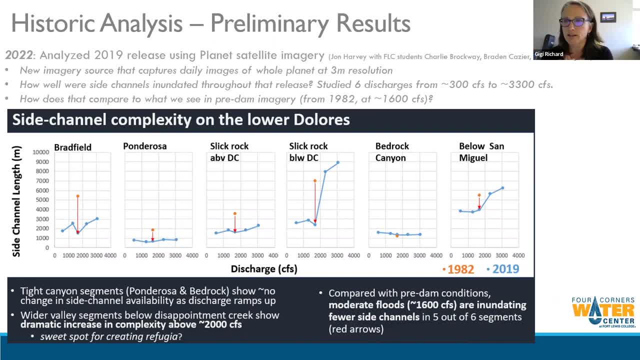 lot of data there. and then salt creek is a new site where blm has been doing some channel clearing. um. so just to share some of the preliminary results, i think this is where things get really interesting. um. dr alan casbrack and dr john harvey at fort louis college have worked with a few of our gis students. 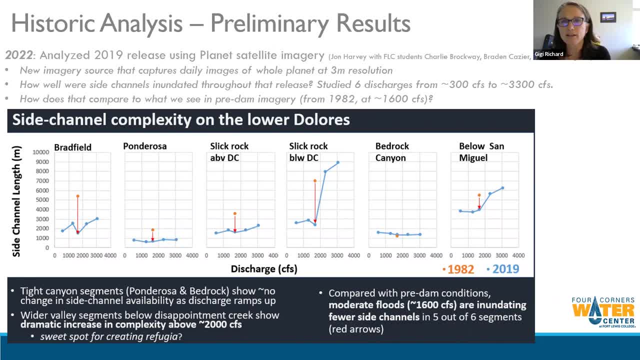 cool resource. there's an organization called planet labs that fly. their satellites are taking pictures of the earth every day, um at three meter resolution. so what they were able to do is go back to the 2019 high flow release and capture um days where there are no clouds. so that's so you might. 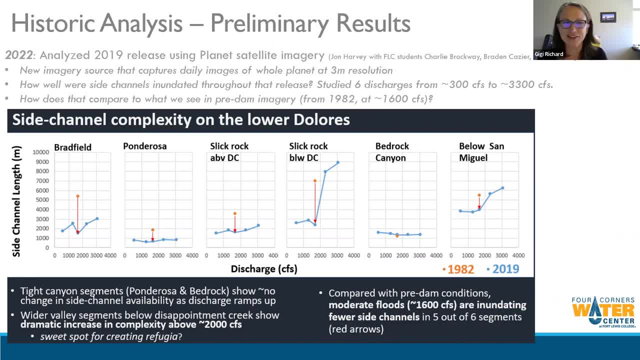 have daily pictures, but there might be clouds every day, so it's not useful. so you have to find cloud free days and find the discharge on those days and then digitize the all of the channels. so the um, planet labs and imagery- and i just realized i didn't include an image in that i'm going to pop. 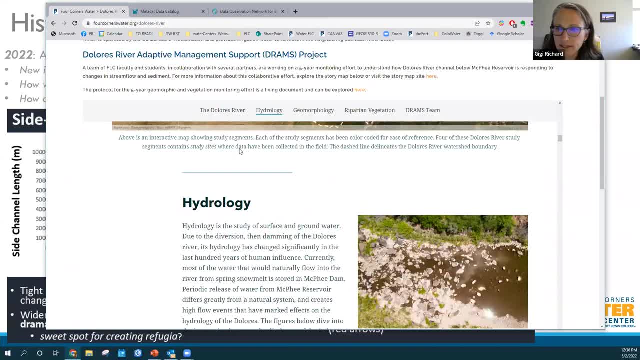 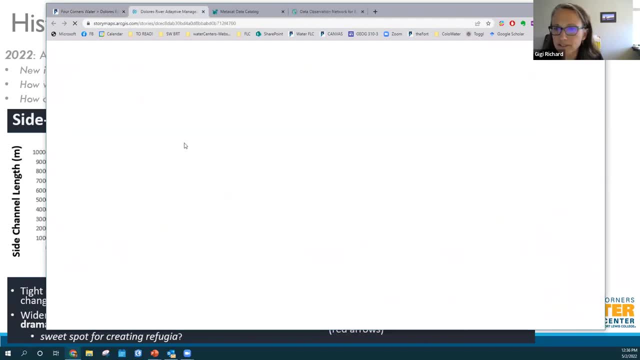 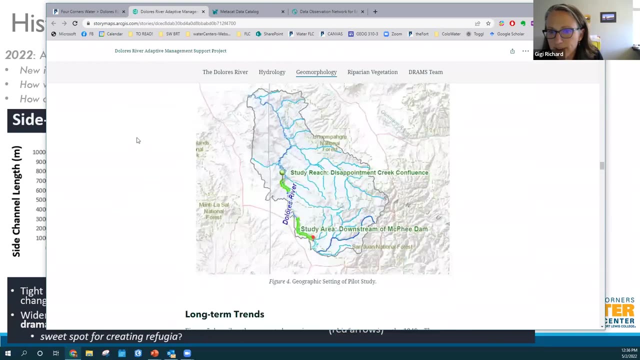 over actually to the website, because in the story map it's actually really cool to see. i'll open up a bigger version of it and you, you to the geomorphology piece. sorry to be scrolling. Here we go, this one I want to show you So. 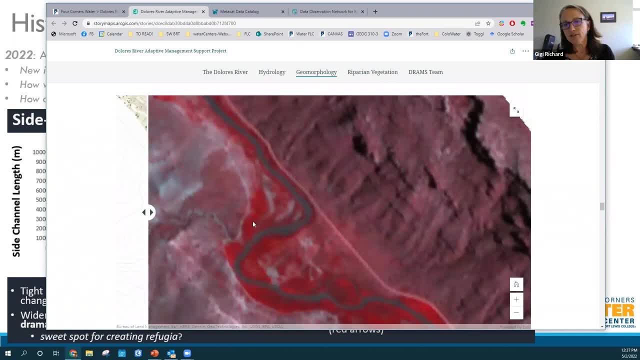 the Planet Labs imagery look like this: They're infrared, so the vegetation shows up as red water shows up as this darker color, so it's really easy to detect where there are channels that have been inundated. And so what they've done is digitized all of the channels, including 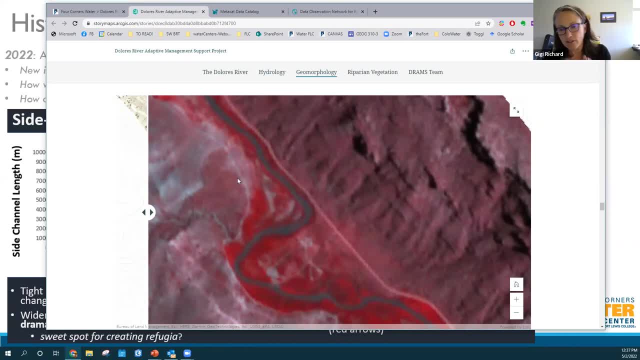 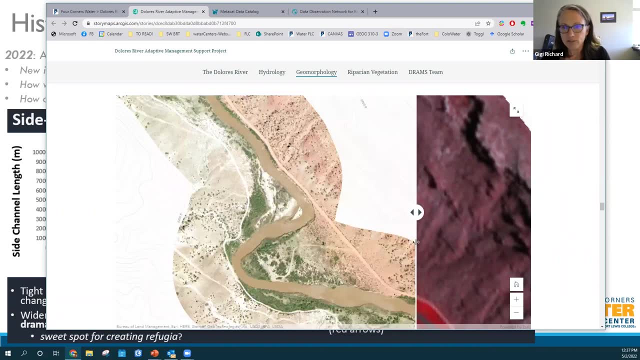 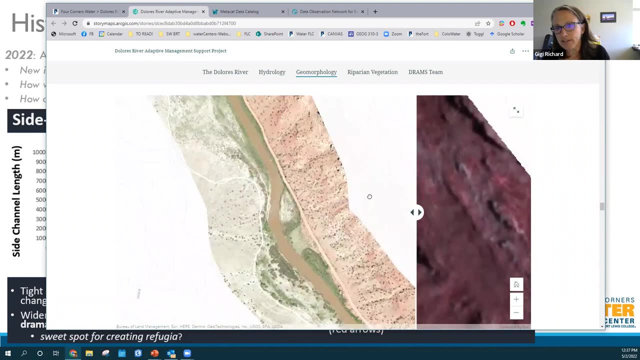 all of the side channels at different discharge levels during the 2019 release. And then they've also done that for 1982, which is pre-McPhee damp, And so this is one of the resources they've created is this ability to swipe back and forth and scroll along the channel. 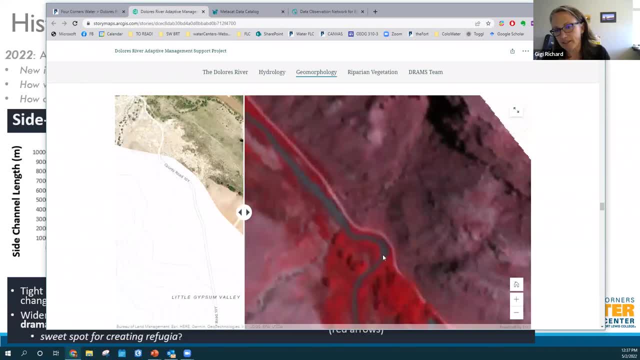 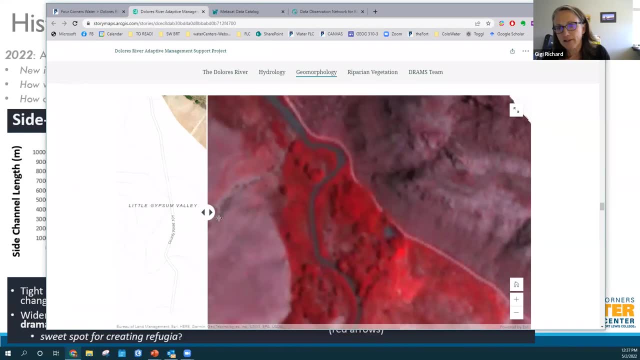 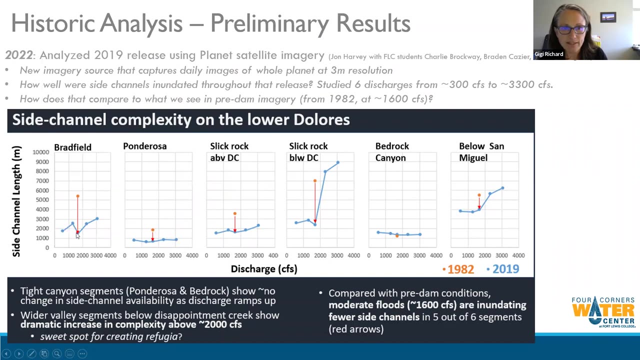 so that we can more readily. you can really clearly see the, the, the encroachment of the vegetation, simplification of the channel and narrowing of the channel. So these results, then, are showing the blue line is 2019 total side channel length at: 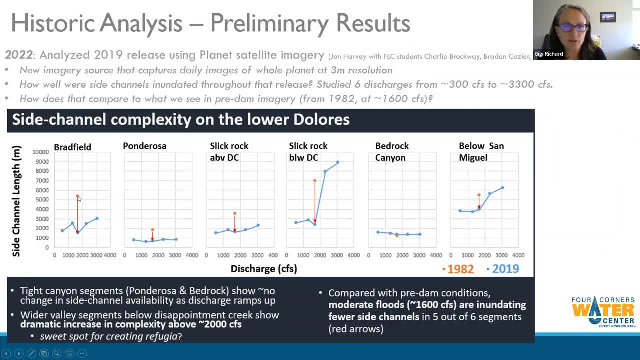 different discharges. The red dot is total side channel length in 1982.. So at all of the sites except Ponderosa is a canyon reach segment and Bedrock Canyon is a canyon segment. at all of the other segments of the river where the river has more ability to move around. 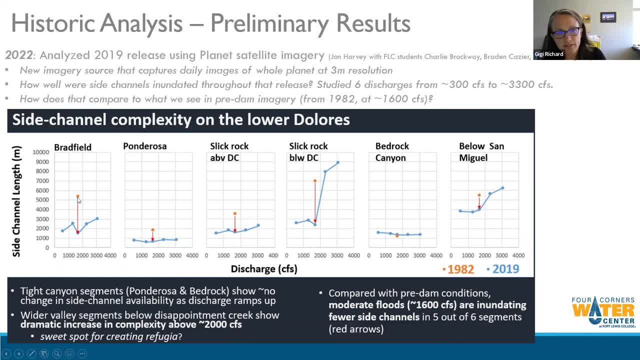 and is where we've seen more changes. we see a reduction in side channel length, And one of the pieces of this that can be really useful for decision making about releases is to look at so, for example, this slick rock site below Disappointment Creek from 1600CFS. 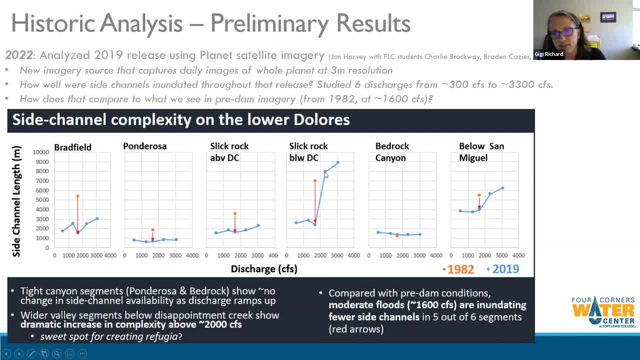 to 2000CFS, we see a really big change in the length of inundated side channels. So in the future, you know thinking about planning releases if we're trying to get more water into side channels, maybe getting to 2000CFS. 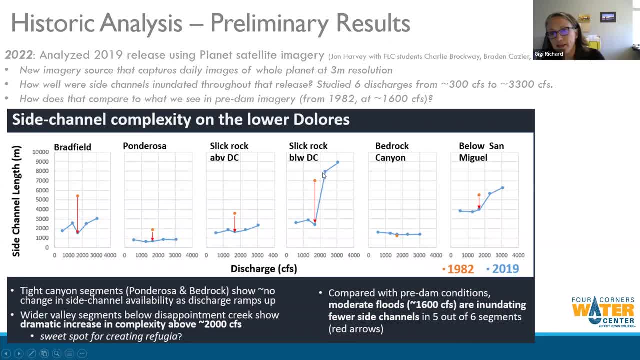 is, should be a sweet spot, a target, whereas maybe getting up then beyond that, to 3000CFS doesn't really give you as much bang for your CFS buck. So so that's the kind of thing we're hoping: to be able to understand more about the channel from this effort. 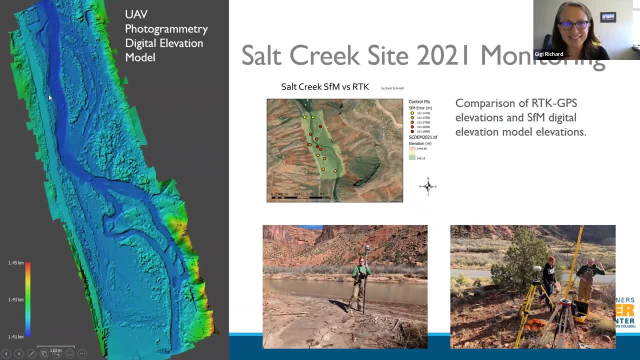 Just to share some of the results with you or some other. the data: this is from Joel Schultes for the Salt Creek Reach. This is downstream of the confluence with the San Miguel, the DEM or digital elevation model that results from their drone flight. These are using structure. 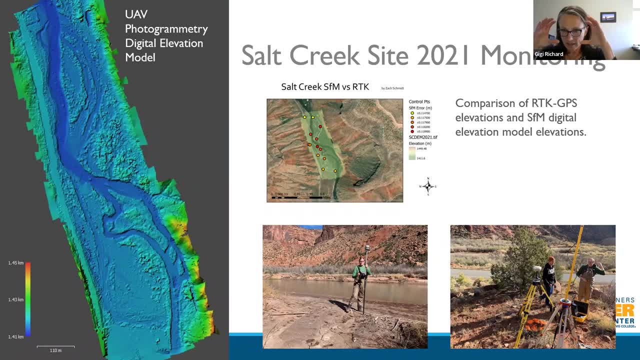 from motion, which is kind of you think of the old USGS elevation that you got from using stereo imagery. So it's the same thing does not remove vegetation, so that has to be dealt with and filtered out. One of the things they're working on is comparing the, the elevation model from the. 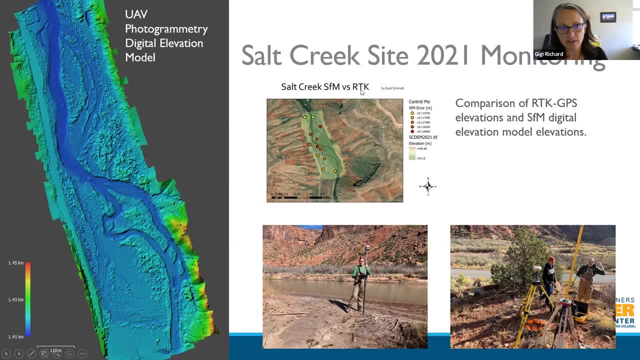 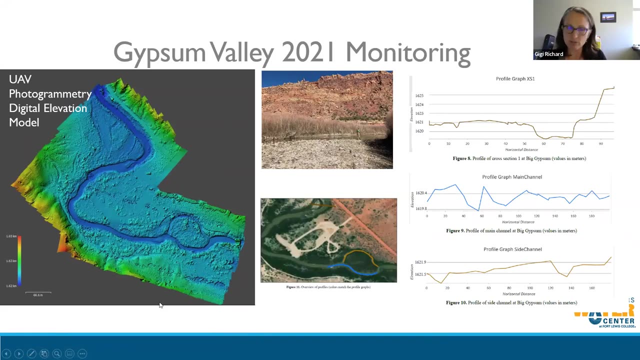 structure from motion with survey grade GPS, RTK, and seeing what sort of accuracy they're getting. So it's about a tenth of a meter at this point with the drone flights, The drone flight of the big gypsum Valley. this is one that's been resurveyed many times with the 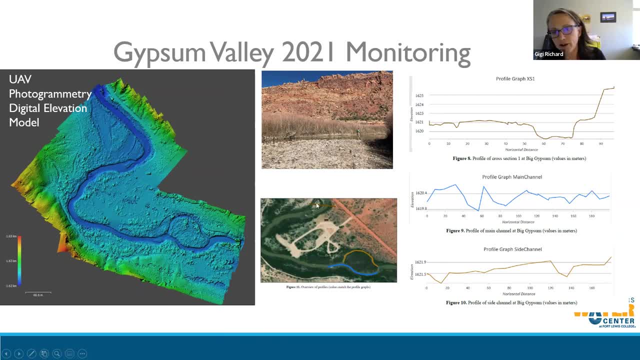 also a lot of fish work there. We also have groundwater monitoring wells on this point bar, So this cross section here is going across that point bar. And then these are two of the profiles are just some of the we haven't. this is all just done in. 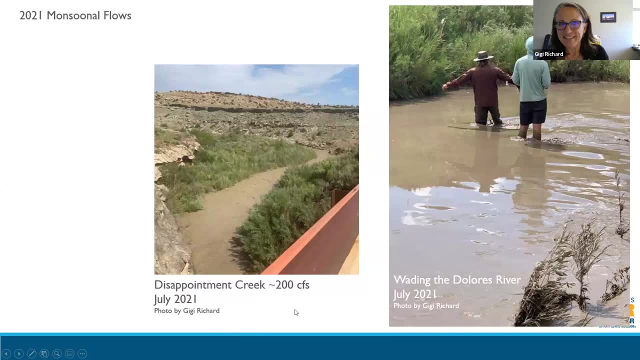 November. So we're there working on processing it now, And this past summer there was very minimal release from McPhee Dam, But we did have a monsoon season and Disappointment Creek, the one I mentioned, that has more sediment than water. 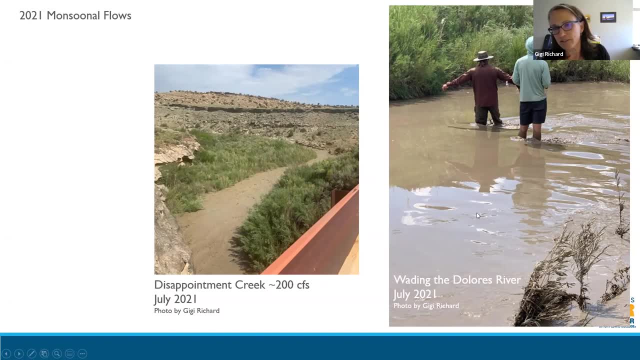 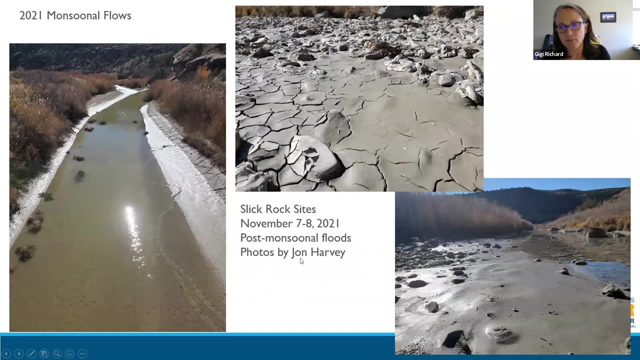 flowed into the Dolores, So this is waiting. across the Dolores River during those monsoonal flows, The deposition of that sediment had a pretty dramatic impact on the channel. John Harvey was out at the slick rock sites following those monsoonal flows in November and you can see the deposition of sediment. 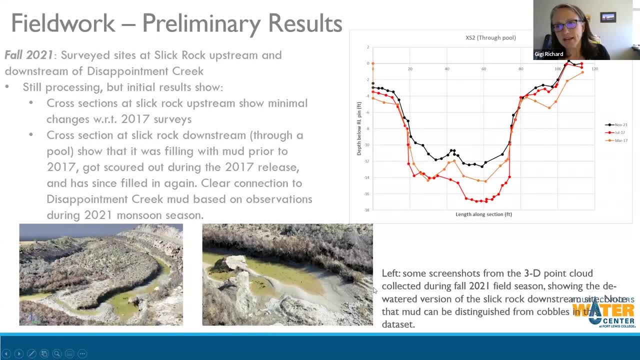 that occurred At that site. they resurveyed a pool that was surveyed pre and post flood in 2017.. And just to give you an idea of what happened there. So here's this orange is March of 2017, the bottom of the 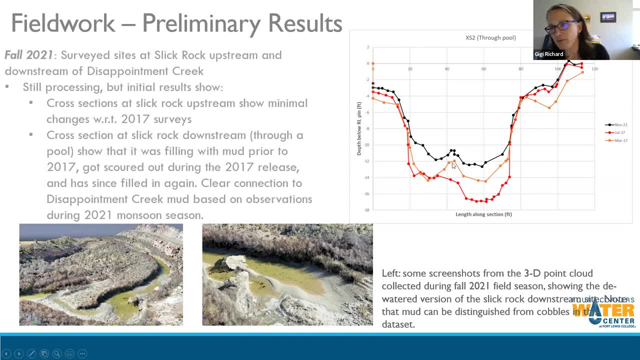 pool. The flow- high flow- of 2017 scoured that pool out, So scoured about three feet of sediment out of that pool And now, in 2021, that pool then has refilled with another about five feet of sediment at the deepest portion. So one of the things 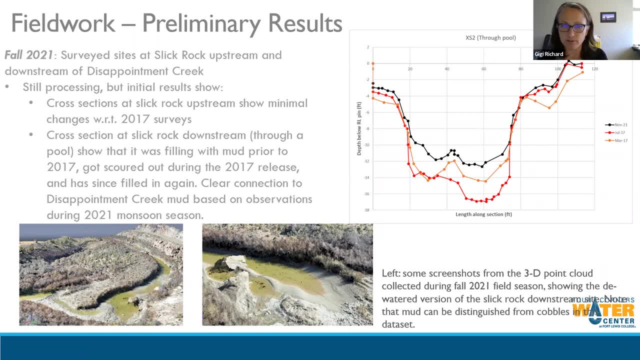 we're learning from this process? is these really low flows, with the monsoonal flows, may have as much of a geomorphic impact as we would anticipate our high flows to have. So not surprising. But as we move into a drier period, we're you know. 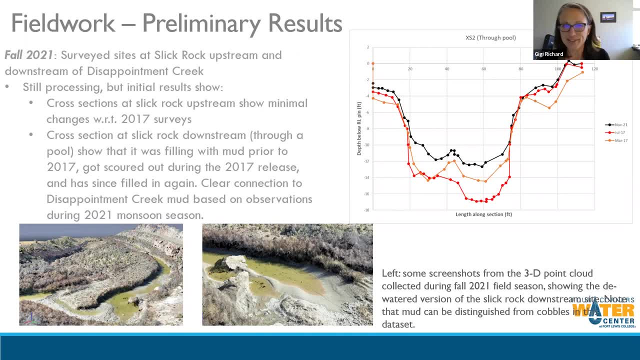 firmly embedded in a solid drought period right now, So these low flows may become more controlling on what's happening in the channel. Oh, and here's some of the 3d results from that structure: for motion drone flights for this rock reach, All right. so then, all of this data. 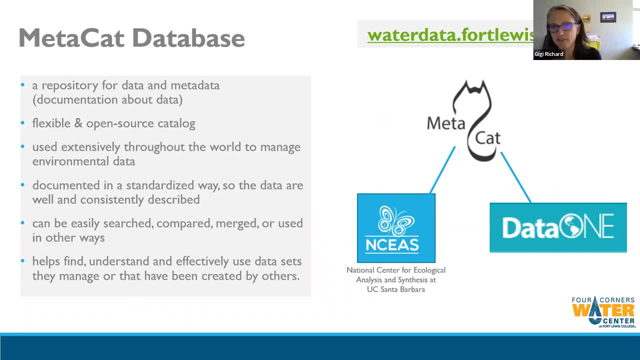 so there's been a lot of work done on the Dolores, So there was some interest in pulling all of this data in from all the different entities who've been collecting it and putting it into a single public repository that would be accessible to everyone, And so we, as part of this grant, we were 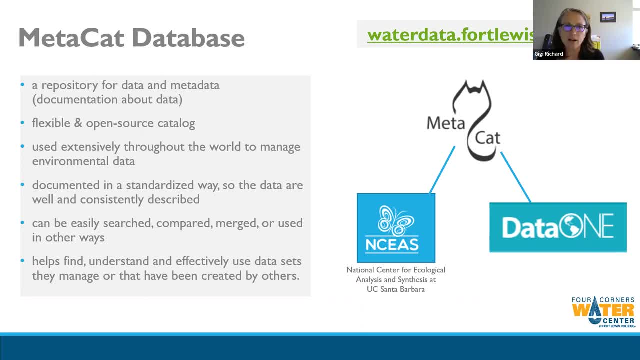 able to pay low to hydrological consultant out of Carbondale to build a MediCat database for us. And we're using MediCat because it's flexible, it's open source And it allows you to document your data, your metadata, your documentation, your data about. 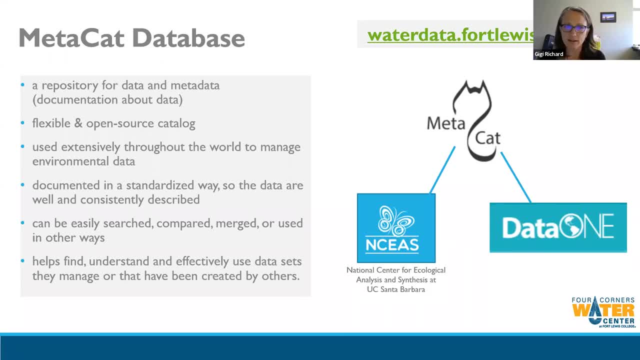 data are all documented in a standard, standardized way, So the data are well described, consistently described, they can easily be searched, compared, merged, used in different ways, And this is the same platform that is used by numerous other databases, such as data one, And there are many. 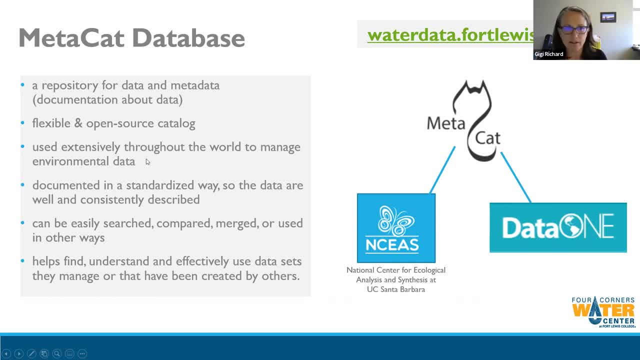 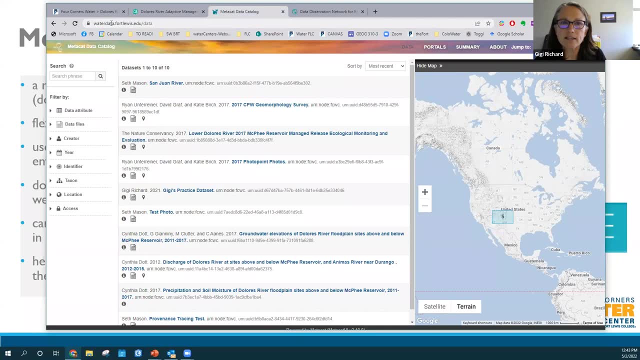 others. hydro share is now using it And there there are others and it's used throughout the world. So I'm just going to pop over here. So if you go to water datafortlewisedu, you'll see that you can go to water datafortlewisedu. that will take. 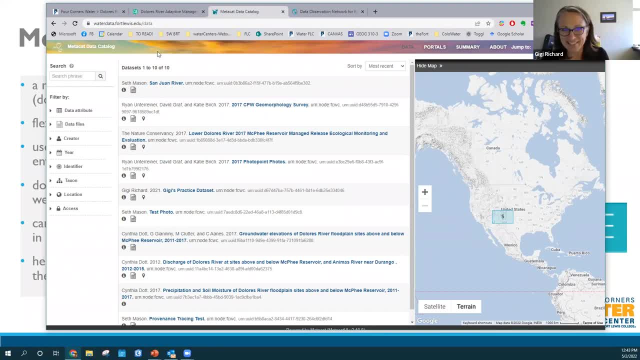 you to the end. this is very much in its infancy And still see like. we still have practice data sets, test photos. So we're just you know. finally, we were able to get this going on the Fort Lewis server, which was a huge undertaking for both Fort. 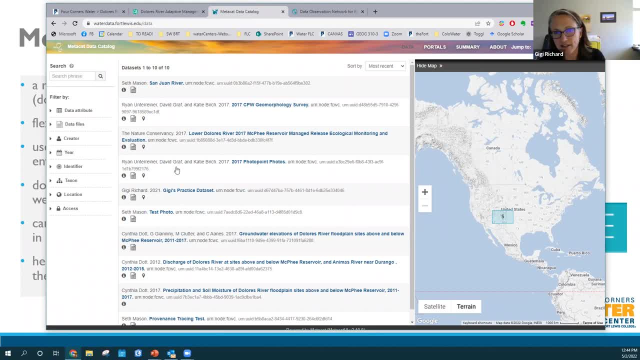 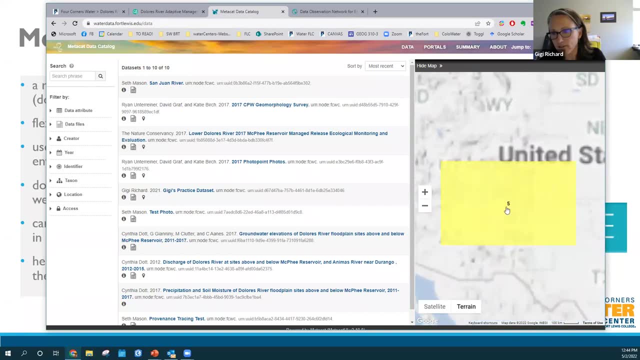 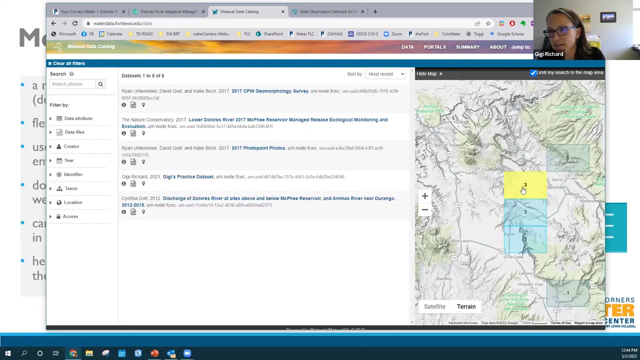 Lewis it and Seth and Bill with Loda hydrological. So, but what we? it's all of the data- have geospatial referencing, so we can zoom in And as you click on a site, it tells you: let's see which one is going to this one. this is our. 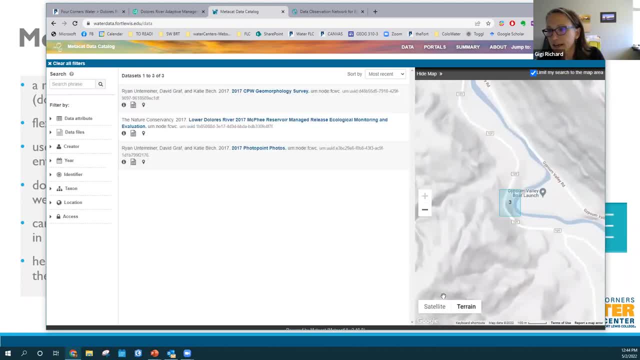 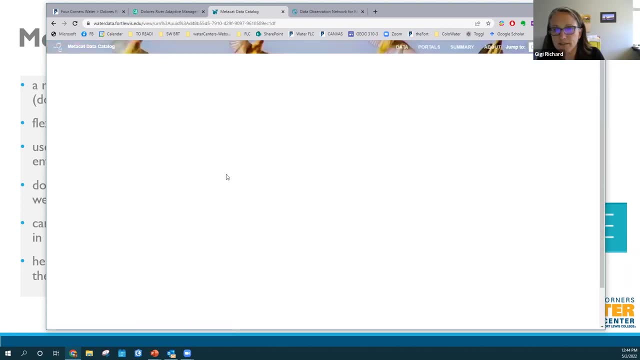 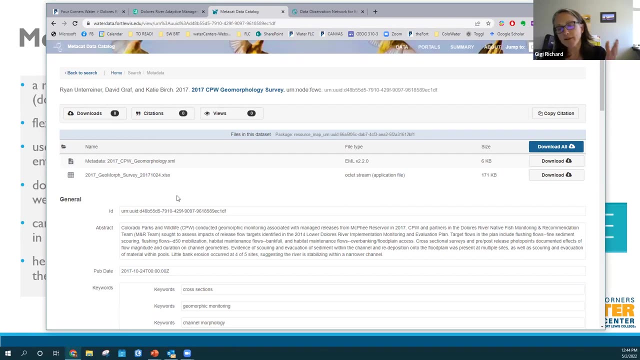 big JIP site. So there are three studies here at the launch And then if you click on one of the studies, you get the data. So in this case it's a spreadsheet. Oh, so one of the other cool things about a MediCat database. 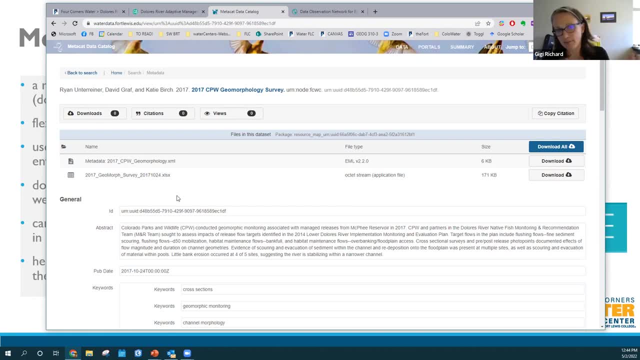 it does allow you to store data of any type, So just PDF, studies, PowerPoints, Excel spreadsheets, GIS data- And it also allows, if you have scripts that run on data that you have used to process your data, you can show the provenance of the raw data. 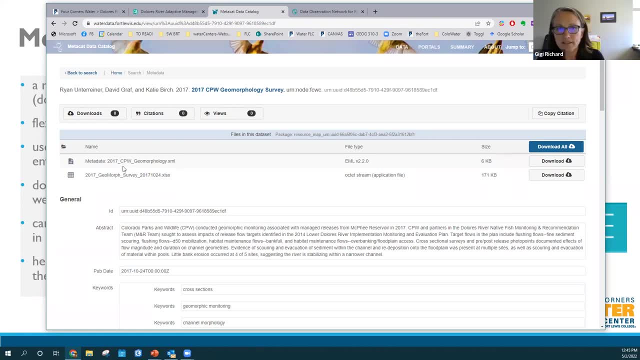 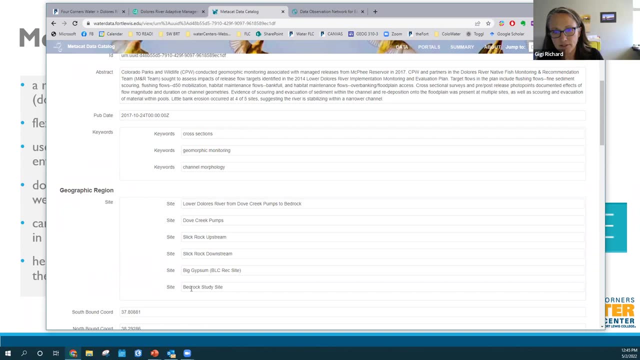 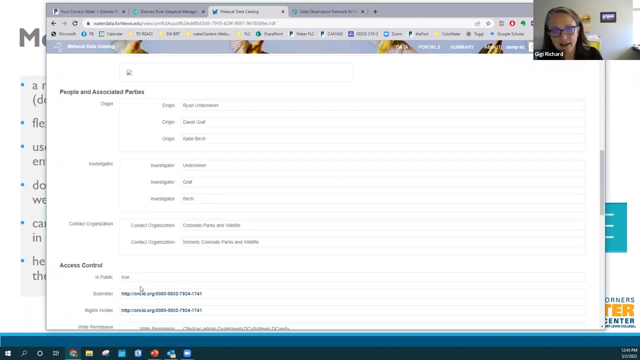 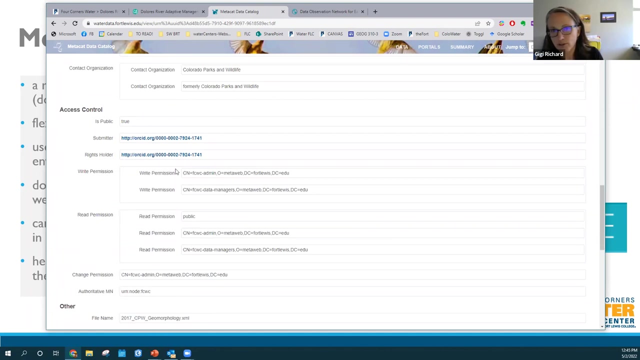 through the processing to the final output. The data can be downloaded. There's an abstract. you have keywords to make it searchable, tied to your study sites. key people who collected the data. who to contact to to if you want to find out who you know. 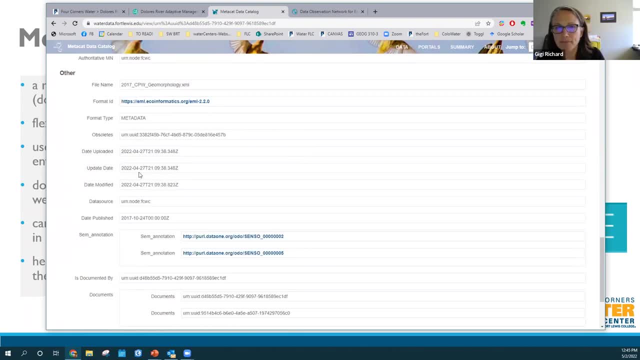 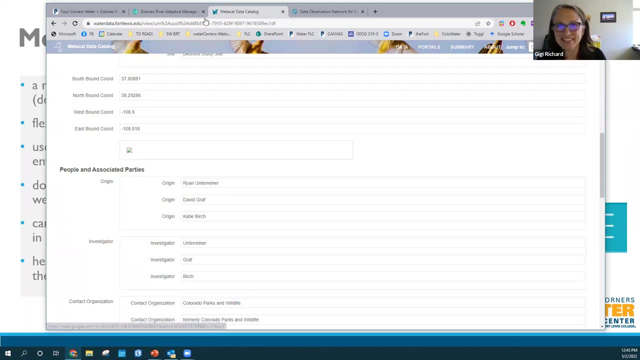 who to contact to get a hold of about the data. We have a lot of work to do to kind of tidy up our metadata to make it all consistent across all of the data. So that's one of the different sources that we have. But I just 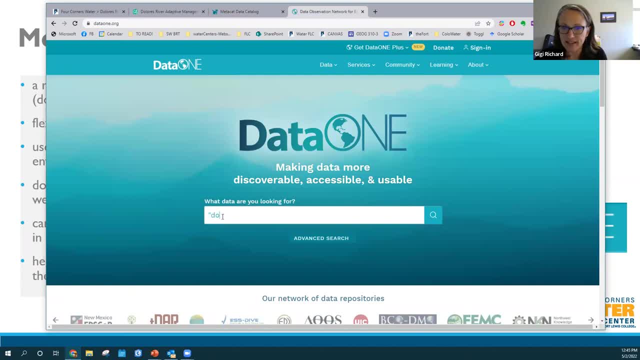 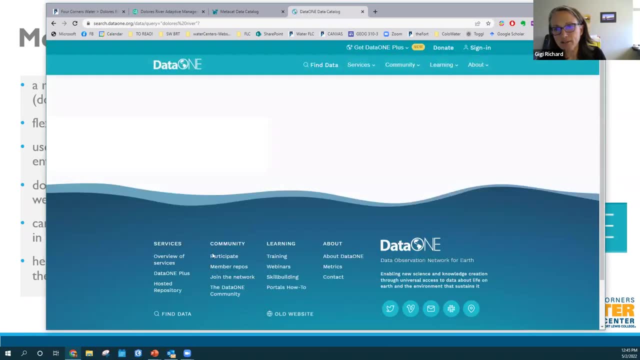 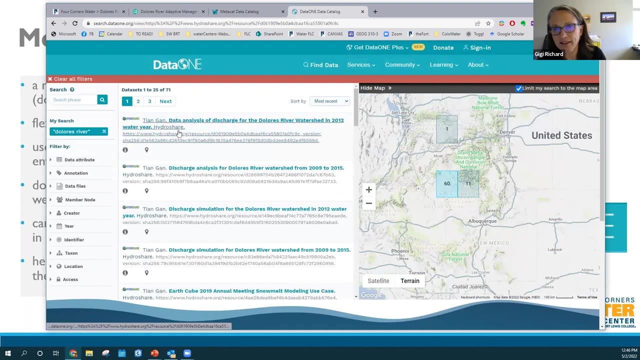 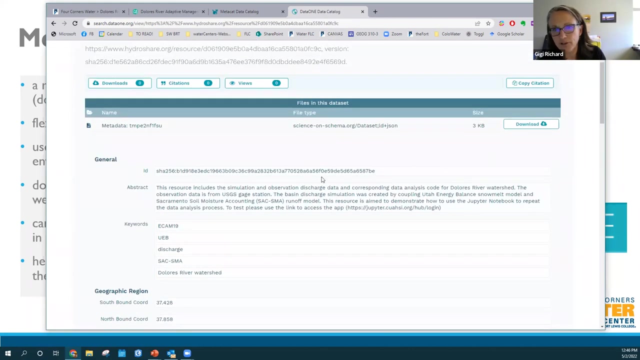 wanted to show you what this full build out looks like. So this is the data one database that ultimately ours will look more like, And so it's searchable And then, and so you can see this really similar format where you can download the data, but then also things are different. So that's one of. 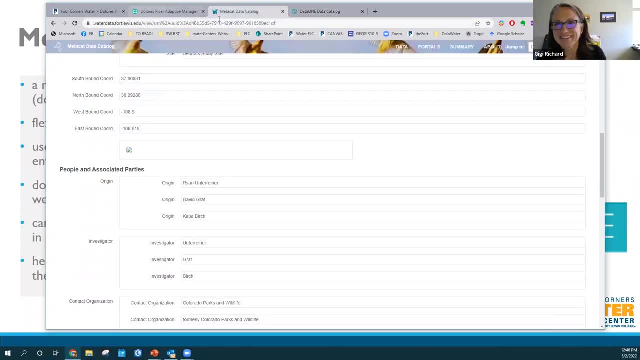 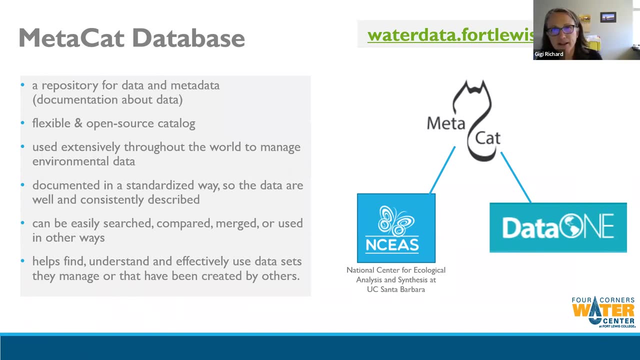 the reasons why we're trying to work with you and that's a really good way to start. That's making sure that the HTML engine and the gh0l do a lot of work. So we're on our way there And hopefully in. 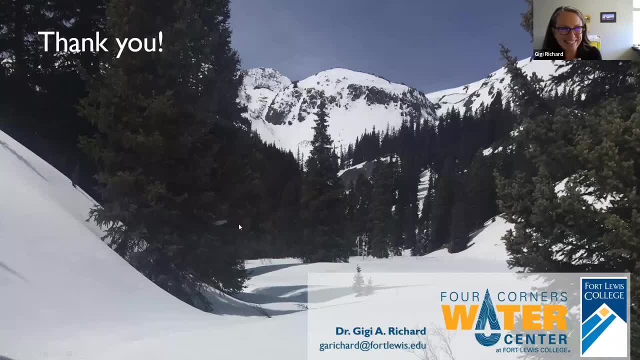 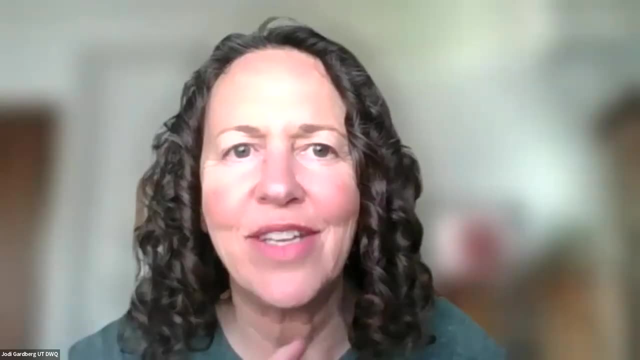 the next couple of months, we'll at least have all of the 2017 studies through present loaded in the database. So okay, so I did it. We have plenty time for q&a if anyone has questions. Awesome thanks. I'm so impressed with the number of partners you have. 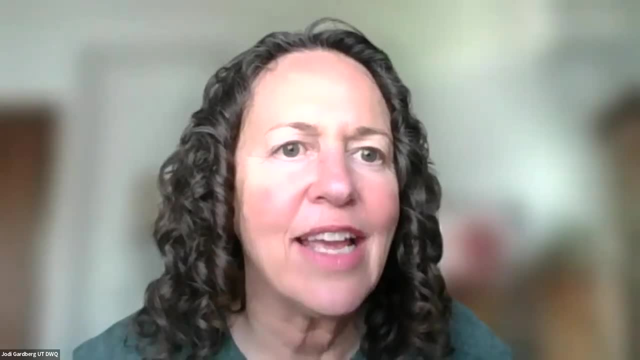 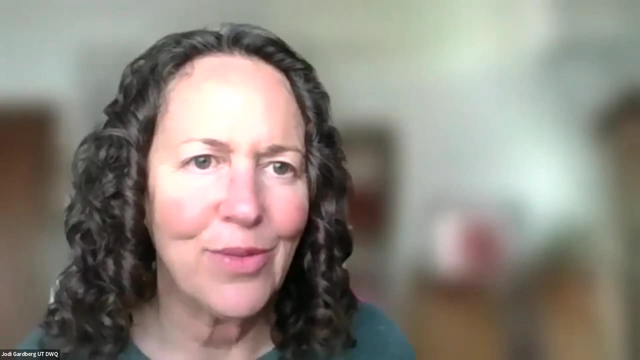 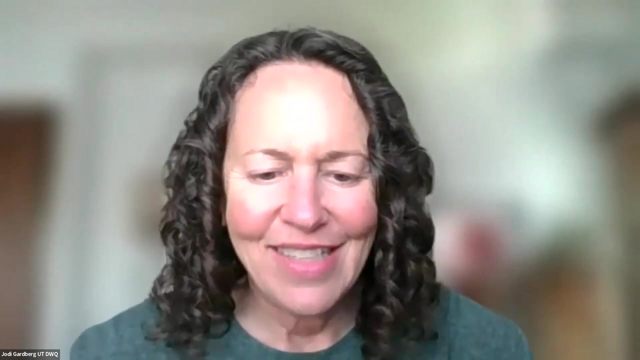 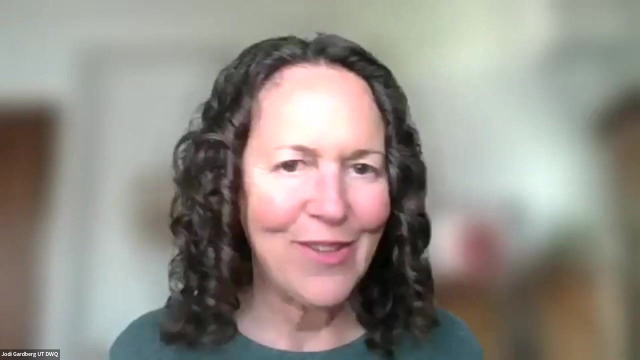 the different types of data that you collect, and then the way it's stored and accessible. So just fantastic work, really, And the mission of the Four Corners Water Center- just so impressive. Thank you, Thank you, Thanks. Yeah, did anybody have any questions for Gigi? 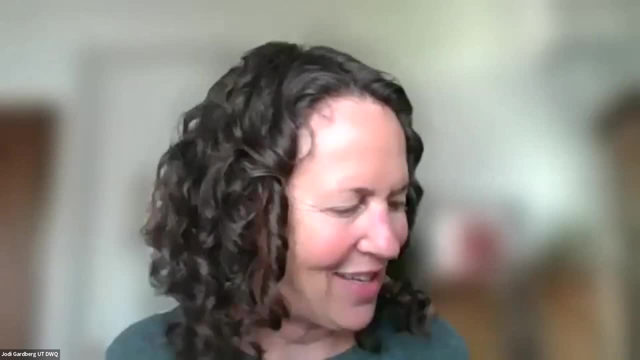 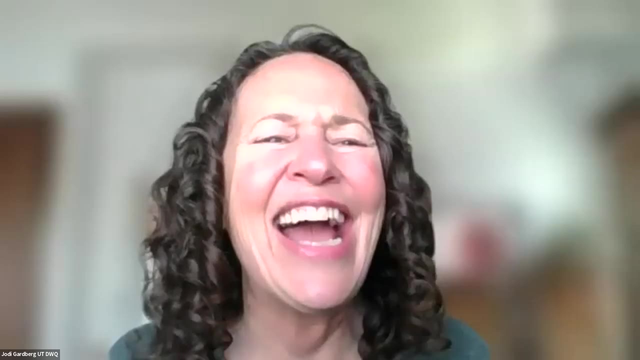 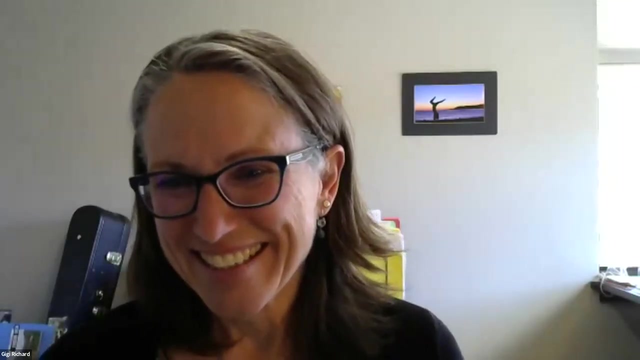 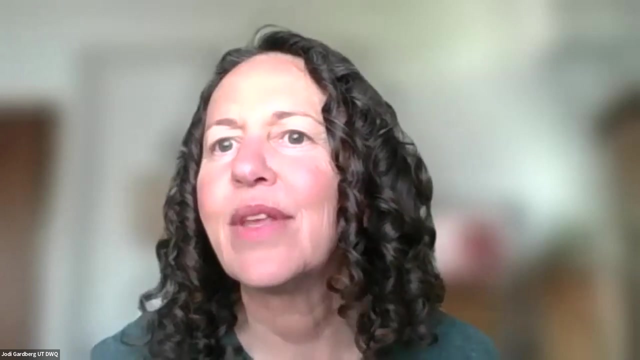 We have a quiet group today At school. we're at that point in the semester where everyone's just Point in the year where, Yeah, I know So Eve Red said incredible, Will the PowerPoint be made available for the group? 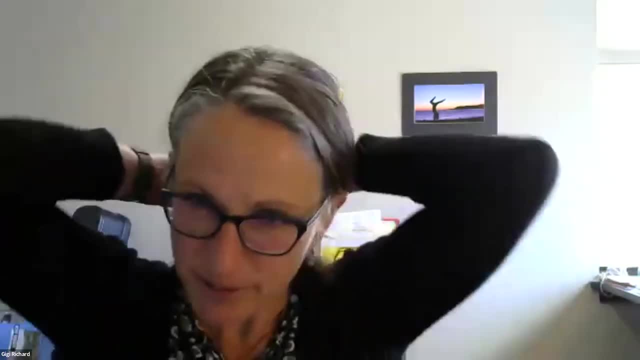 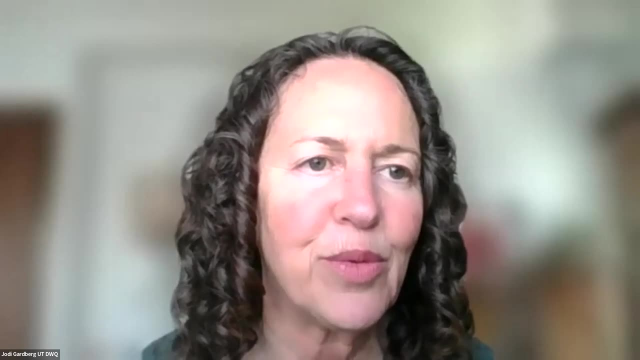 It can be Sure. Oh good, Thank you, Or? I think you're recording it too, aren't you? Yes, we are Send it to Carolyn Gillette or to Christine and I, and we'll post it, OK. 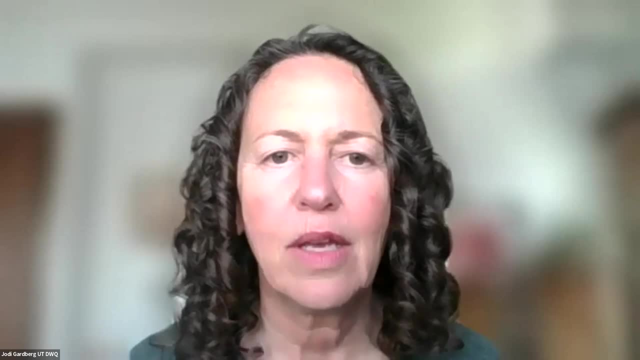 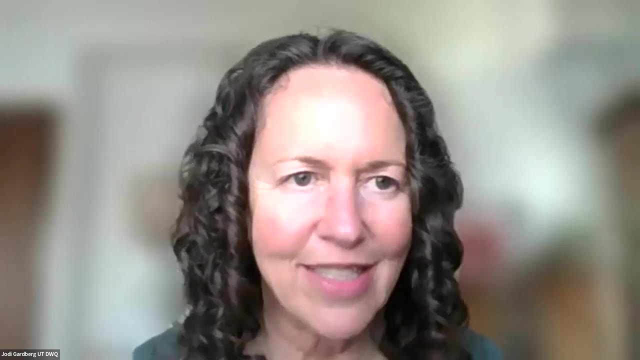 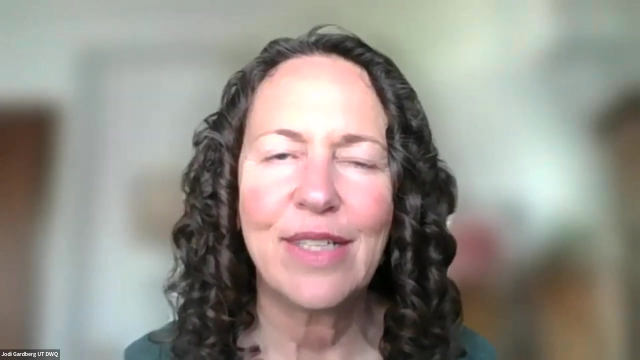 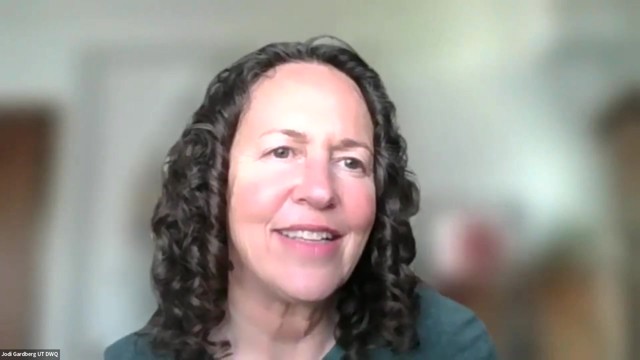 Yeah, Well, I'm going to go look up MediCat database because that was a great way to store your data And we're exploring. do you use high-frequency data in that database? Do you take high-frequency data? Yeah, I didn't think I saw that. 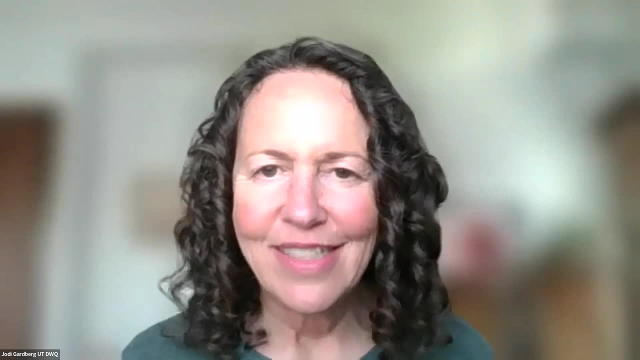 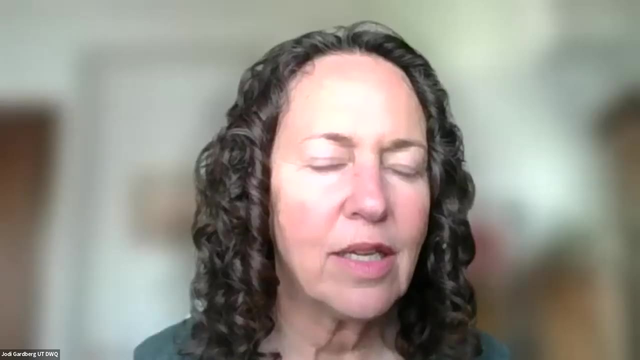 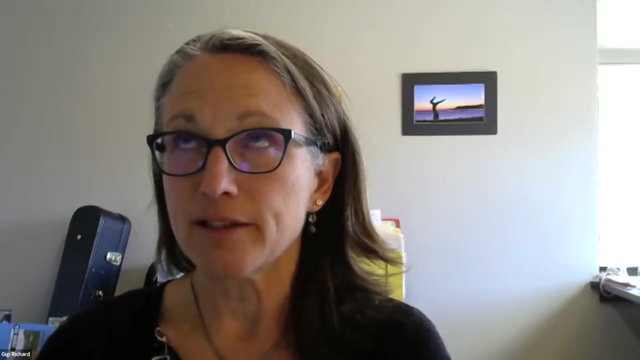 Well, that's what we're exploring right now. Yeah, I get the impression that MediCat is really powerful. Oh good, It does take a little programming on the back end, And in the future we'll hopefully have them build some data entry forms for us. that will make it. 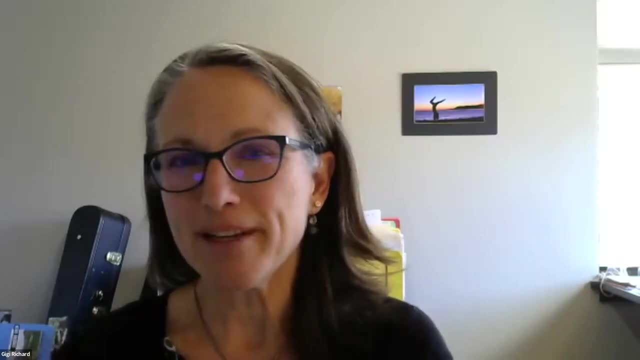 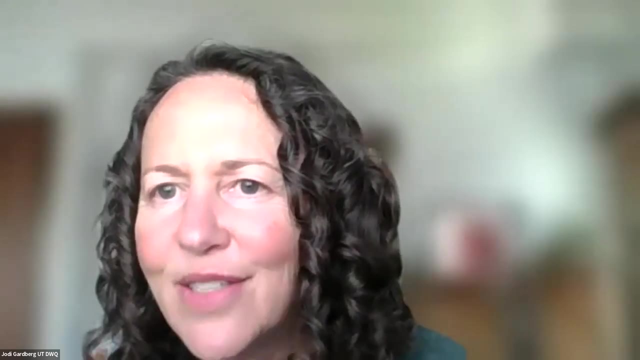 a little more streamlined for the data entry, But I mean, I've already been playing around in it and it's pretty straightforward. Yeah, Excited about that. Someone asked a question: Are there any plans to increase snow level monitoring in the transition area? 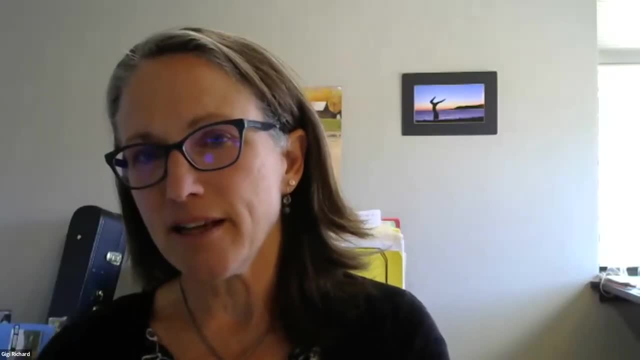 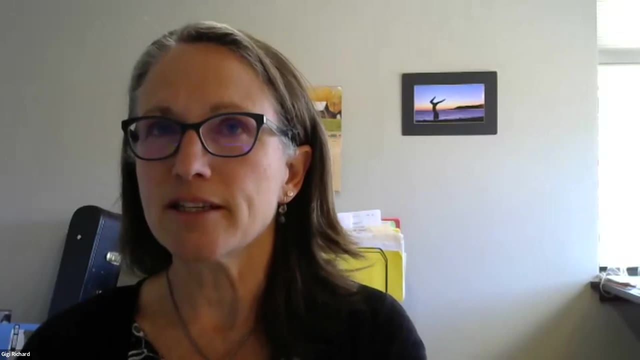 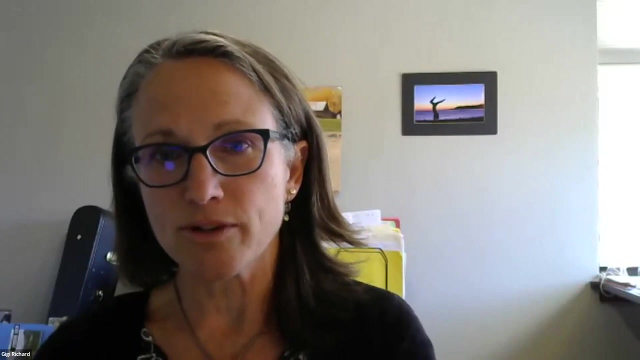 That's a great question. So not with our project. but there is another effort- It has a little bit different focus happening in the Dolores Basin. Well, actually it's in the Chicken Creek watershed With the Dolores Watershed. Resilient Forest- Dwarf. 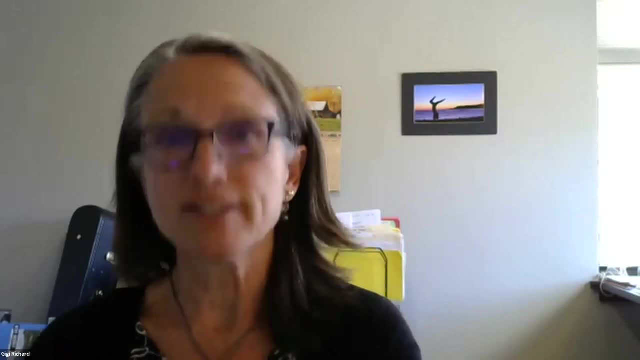 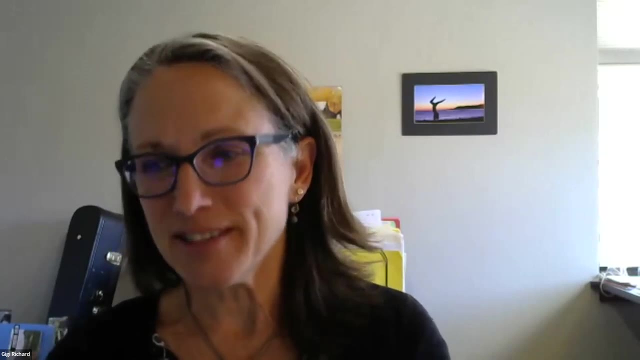 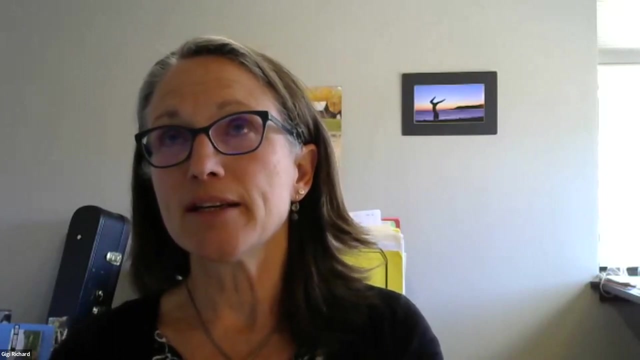 the Dolores Watershed Resilient Forest Collaborative And they're calling this. they call it snowtography And similar thing. they're using the wildlife cameras But they're trying to understand accumulation of snow in areas of the forest that 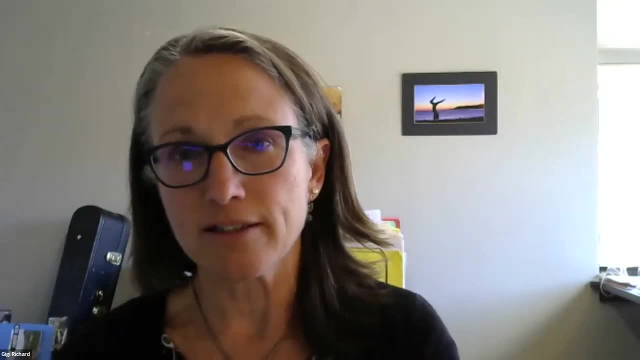 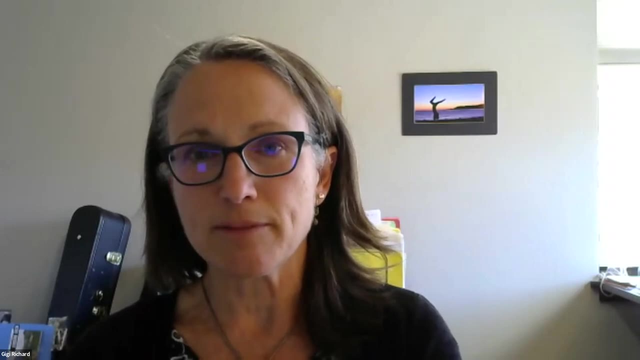 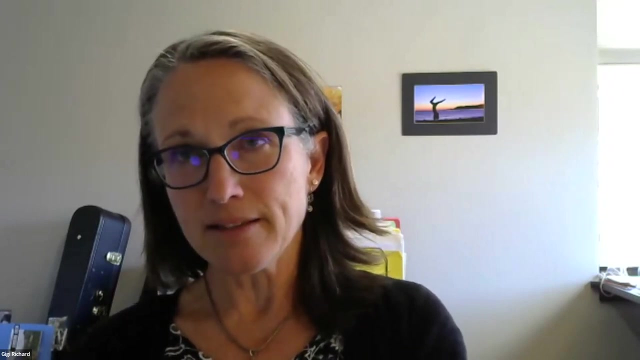 have been treated for fire mitigation versus areas that are not, And I Just on email there. they actually got some more funding to expand that And it's much more in-depth snow monitoring And like six cameras per site with 26 stakes per site. 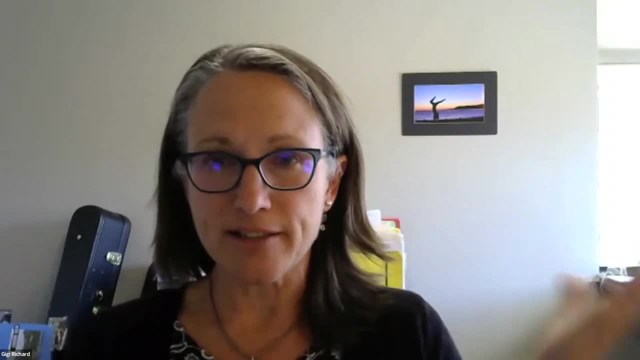 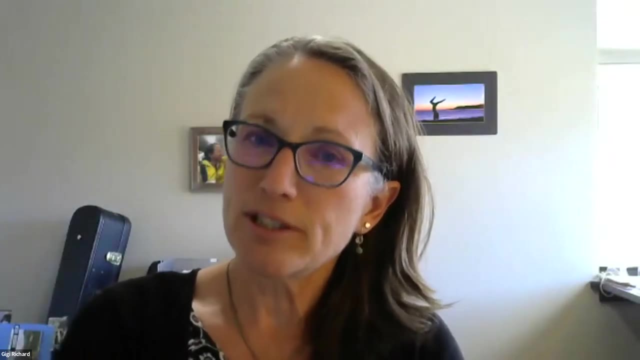 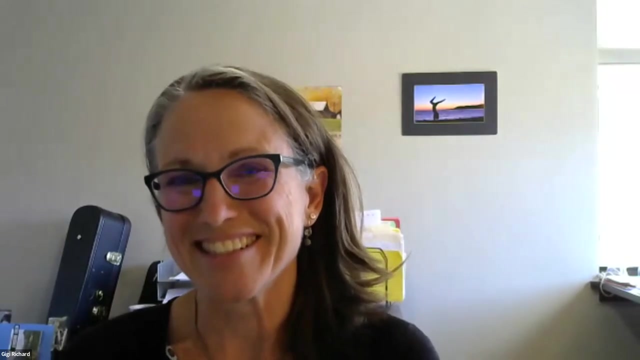 So they have transects of snow depth that measure in the treated area and in the untreated area, And so, for example, the student I have working on the machine learning to process the imagery. those are going to be really But that will be really valuable with all of the images. 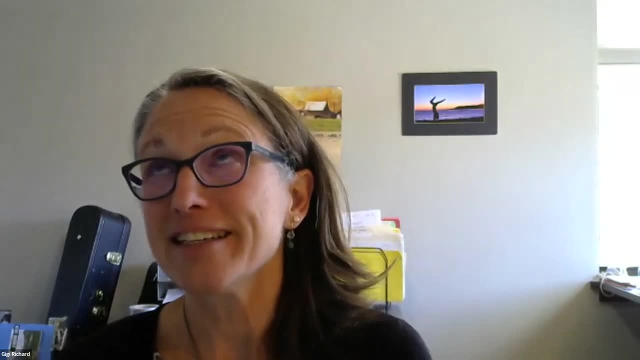 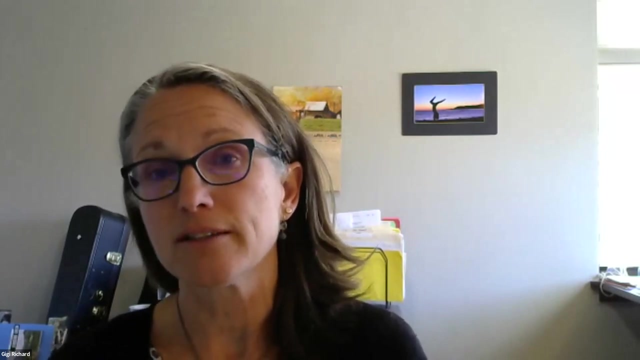 that they have to process. So that's all that I know of. for additional snow monitoring that's happening right now. Yeah, they don't have it paired with stream gauges though, So they're much more. they do have. they're measuring soil moisture and snow.